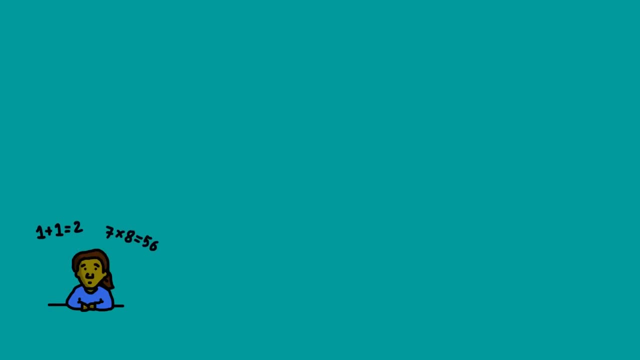 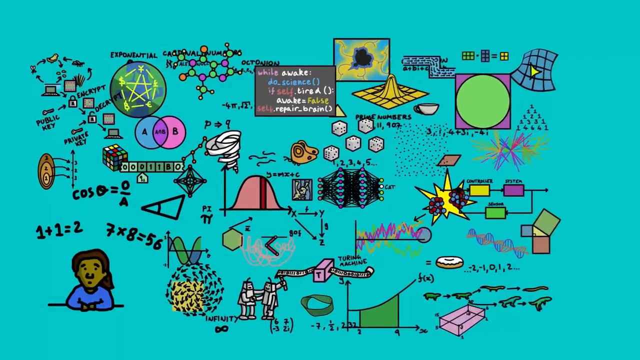 The mathematics we learn in school doesn't quite do the field of mathematics justice. We only get a glimpse at one corner of it. but mathematics as a whole is a huge and wonderfully diverse subject. My aim with this video is to show you all of that amazing stuff. 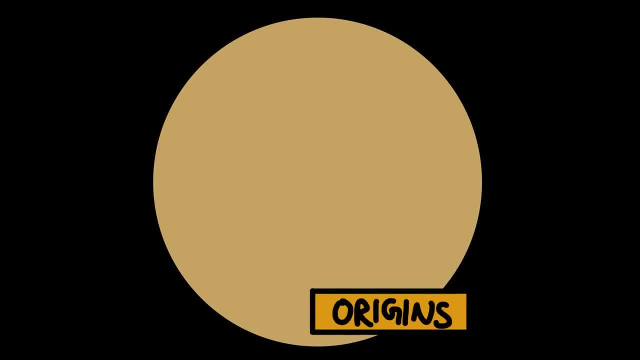 We'll start back at the very beginning. The origin of mathematics lies in counting. In fact, counting is not just a human trait. other animals are able to count as well, And evidence for human counting goes back to prehistoric times, with check marks made in bones. 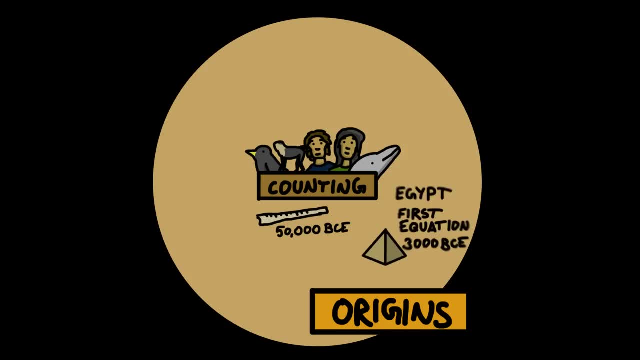 There were several innovations over the years, with the Egyptians having the first equation, the ancient Greeks making strides in many areas like geometry and numerology, and negative numbers were invented in China, and zero as a number was first used in India. Then, in the golden age of Islam, Persian mathematicians made further strides. 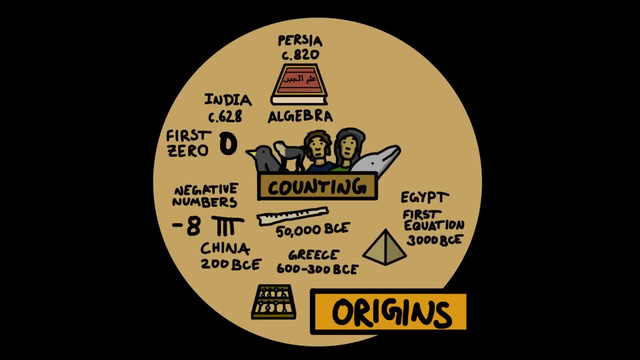 and the first book on algebra was written. Then mathematics boomed in the Renaissance, along with the Scythians and the Romans. Now there's a lot more to the history of mathematics than what I've just said, but I'm going to jump to the modern age and mathematics as we know it now. 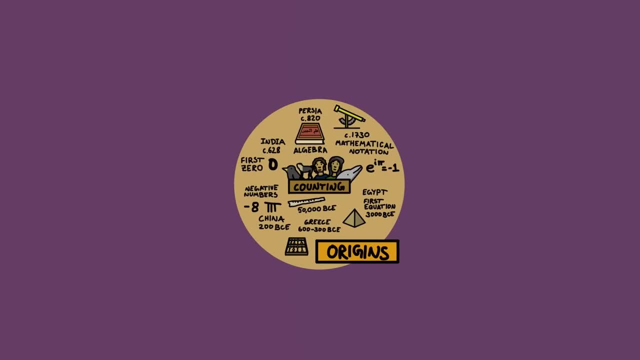 Modern mathematics can broadly be broken down into two areas: Pure maths, the study of mathematics for its own sake, and applied maths, when you develop mathematics to help solve some real-world problem. But there's a lot of crossover, In fact many times in history. 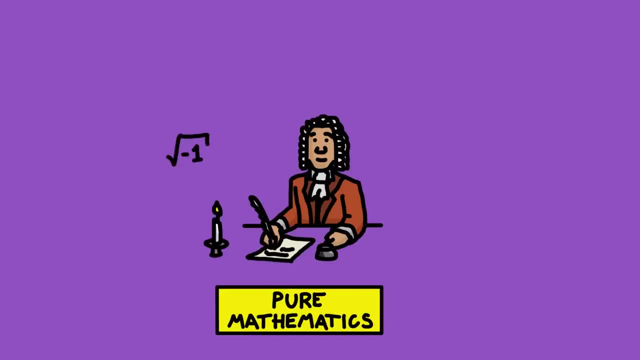 someone's gone off into the mathematical wilderness motivated purely by curiosity and kind of guided by other people's ideas, And that's what I'm going to talk about today. Now I'm going to talk about some of the things that have happened over the last few centuries. 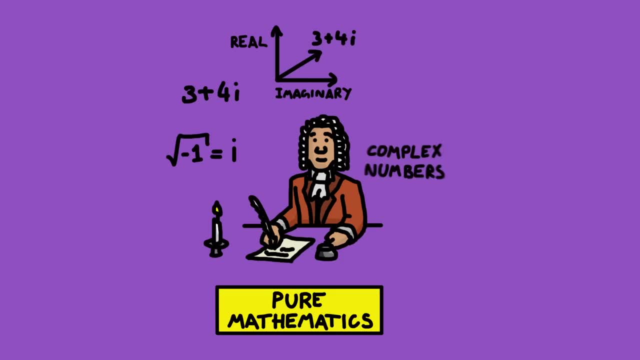 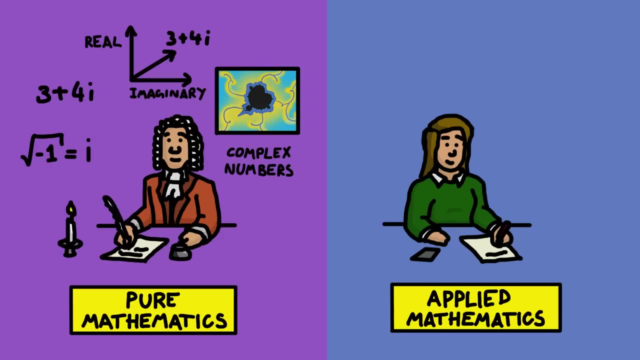 And then they've created a whole bunch of new mathematics which is nice and interesting, but it doesn't really do anything useful. But then say, a hundred years later someone will be working on some problem at the cutting edge of physics or computer science. 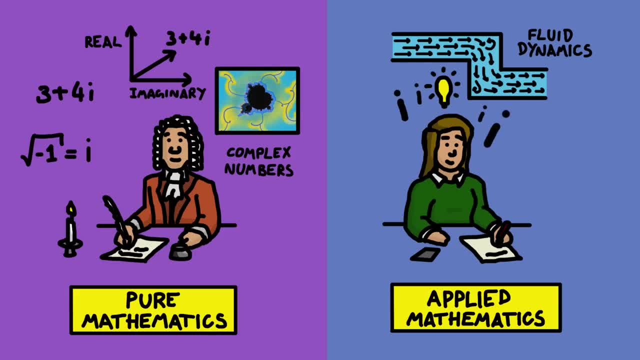 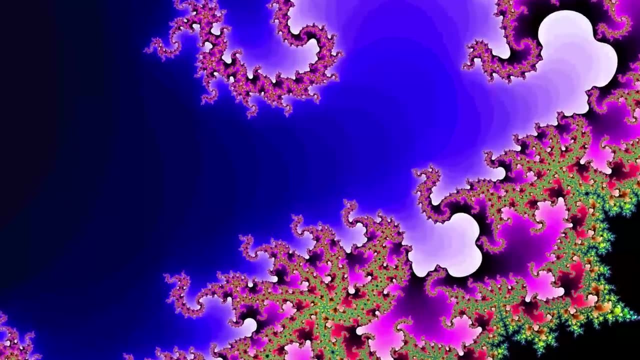 and they'll discover that this old theory in pure math is exactly what they need to solve their real-world problems, Which is amazing, I think, And this kind of thing has happened so many times over the last few centuries. it's interesting how often something so abstract ends up being really useful. But I should also mention that pure 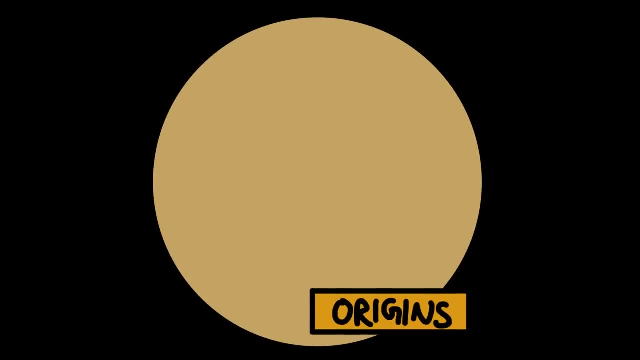 We'll start back at the very beginning. The origin of mathematics lies in counting. In fact, counting is not just a human trait, other animals are able to count as well. And evidence for human 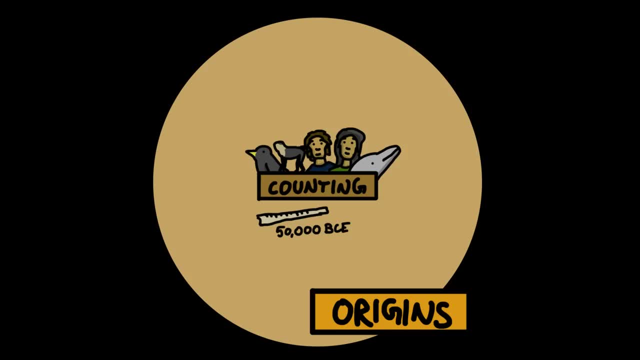 counting goes back to prehistoric times with checkmarks made in bones. 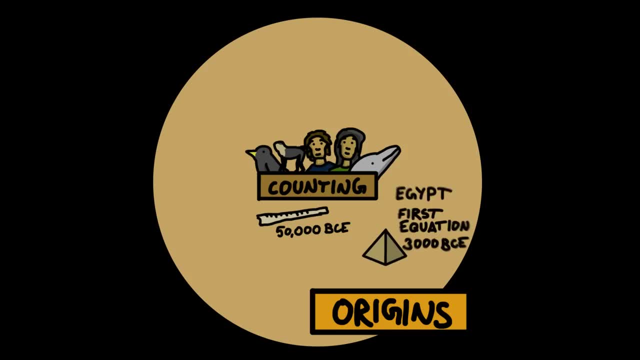 There were several innovations over the years with the Egyptians having the first equation, the ancient Greeks making strides in many areas like geometry and numerology, negative numbers were invented in China, and zero as a number was first used in India. 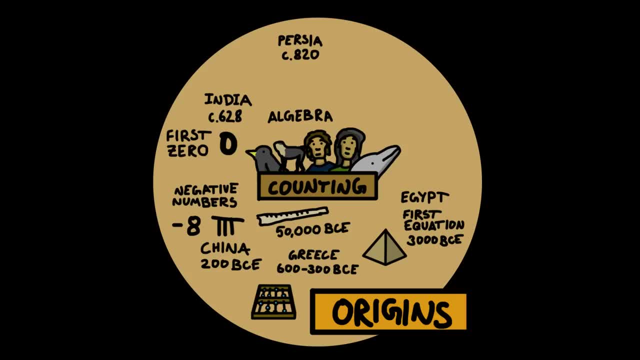 Then in the golden age of Islam, Persian mathematicians made further strides and 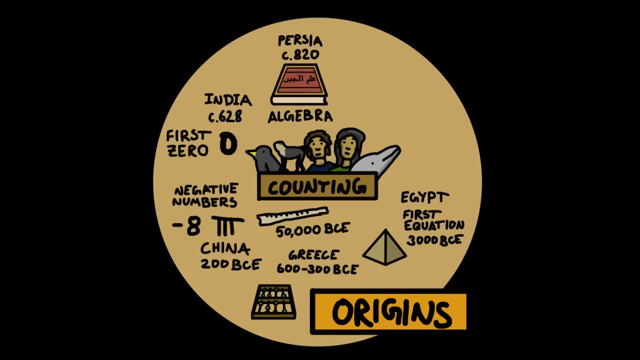 the first book on algebra was written. Then mathematics boomed in the Renaissance along with the Cypriot era. The first book on algebra was written. Then mathematics boomed in the Renaissance along with the Cypriot era. Then mathematics boomed in the Renaissance along with the Cypriot era. Then mathematics boomed in the Renaissance along with the Cypriot era. Now there's a lot more to the history of mathematics than what I've just said, 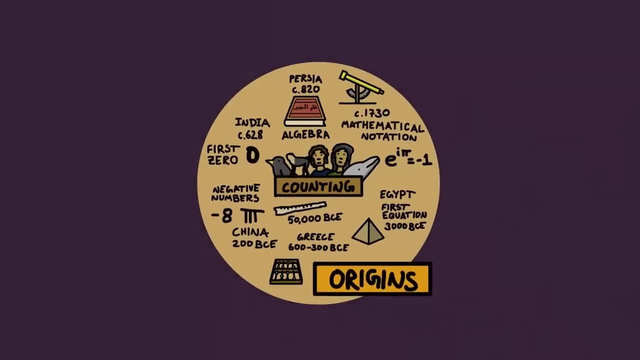 but I'm going to jump to the modern age and mathematics as we know it now. 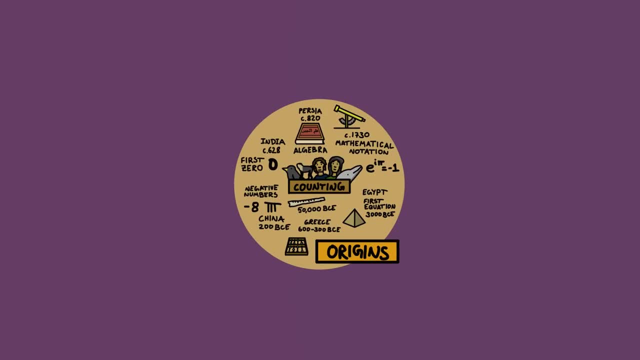 Modern mathematics can broadly be broken down into two areas, pure maths, the study of mathematics for its own sake, and applied maths, when you develop mathematics to help solve some real world 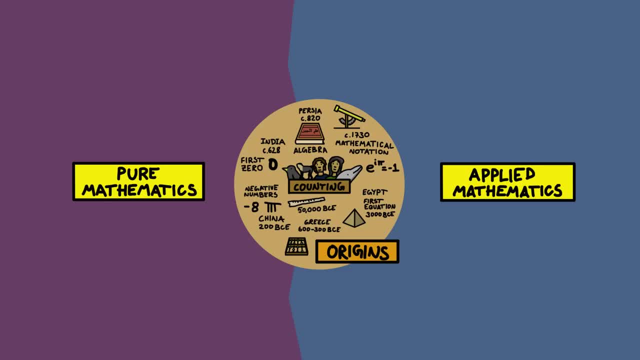 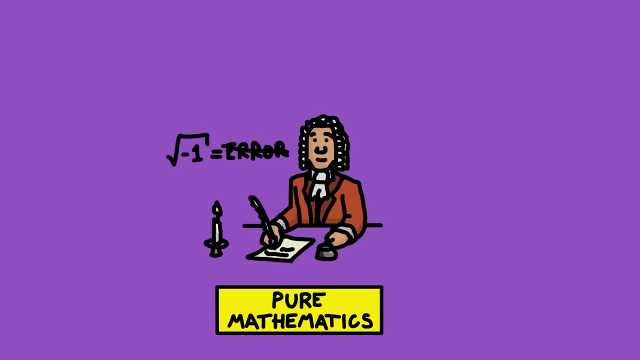 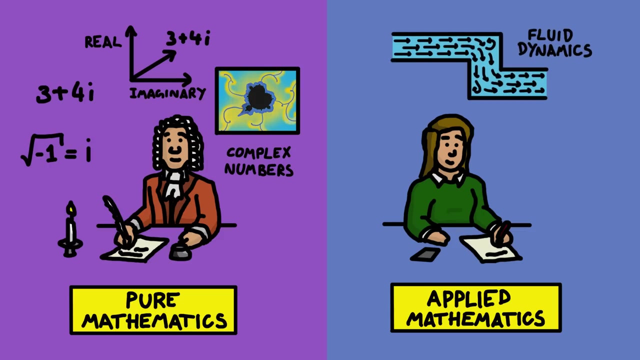 problem. But there's a lot of crossover. In fact, many times in history, someone's gone off into the mathematical wilderness motivated purely by curiosity and kind of guided by a sense of aesthetics. And then they've created a whole bunch of new mathematics, which is nice and interesting, but it doesn't really do anything useful. But then say a hundred years later, someone will be working on some problem at the cutting edge of physics or computer science, and they'll discover that this old theory in pure math is exactly what they need to 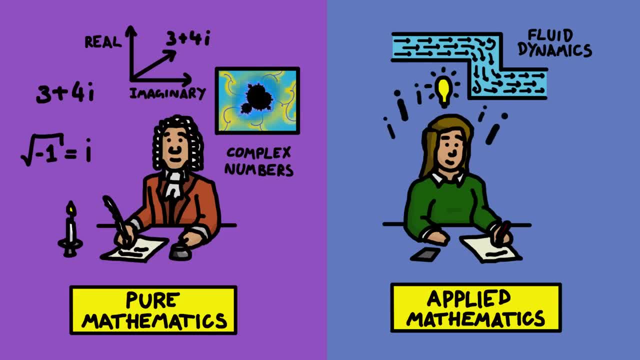 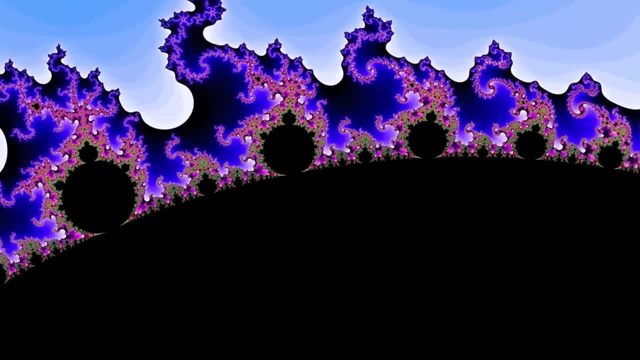 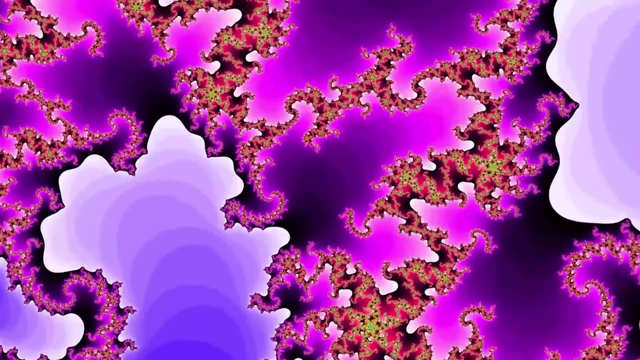 solve their real world problems, which is amazing, I think. And this kind of thing has happened so many times over the last few centuries. It's interesting how often something so abstract ends up being really useful. But I should also mention that pure mathematics on its own is still a very valuable thing to do because it can be fascinating and on 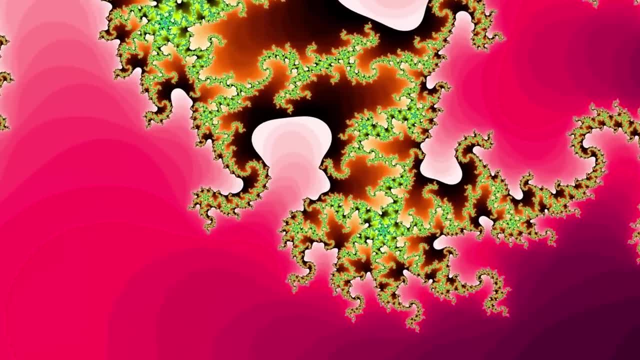 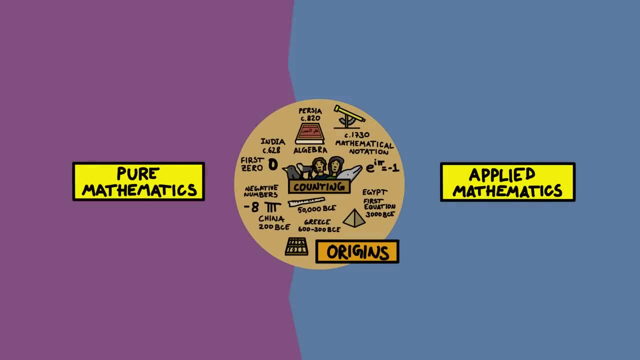 its own can have a real beauty and elegance that almost becomes like art. Okay, enough of this highfalutin. Let's get into it. Pure maths is made of several sections. 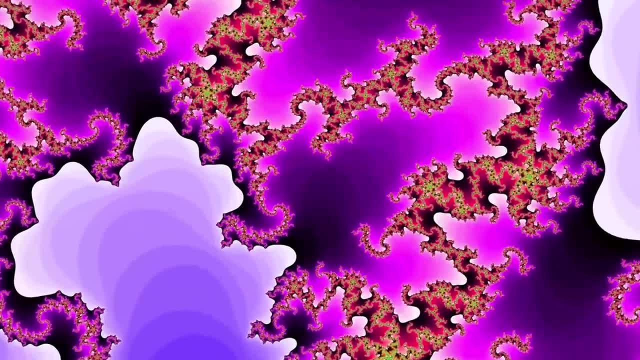 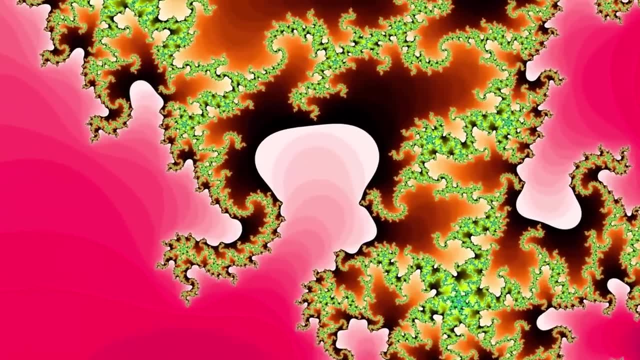 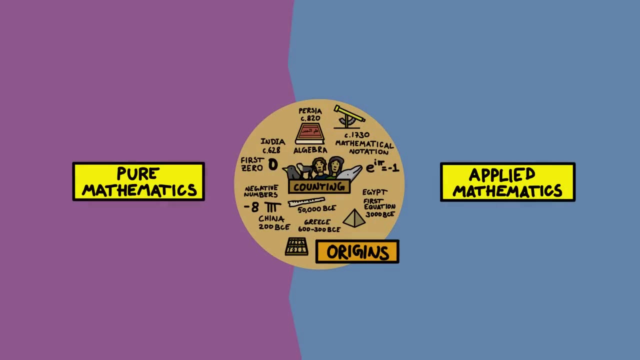 mathematics on its own is still a very valuable thing to do, because it can be fascinating and on its own can have a real beauty and elegance that almost becomes like art. Okay, enough of this hypholutin, Let's get into it. Pure maths is made of several sections. 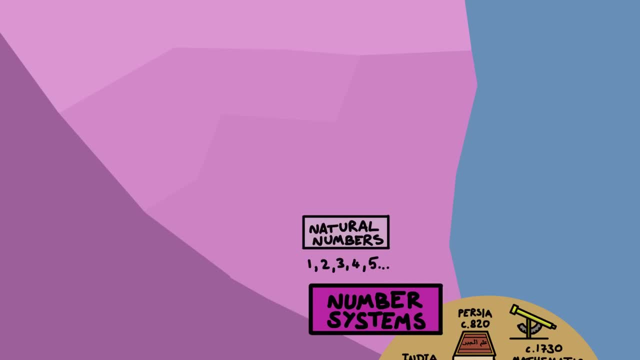 The study of numbers starts with the natural numbers and what you can do with them, with arithmetic operations, And then it looks at other kinds of numbers, like integers, which contain negative numbers, rational numbers like fractions, real numbers which include numbers like pi, which go off to infinite decimal points. 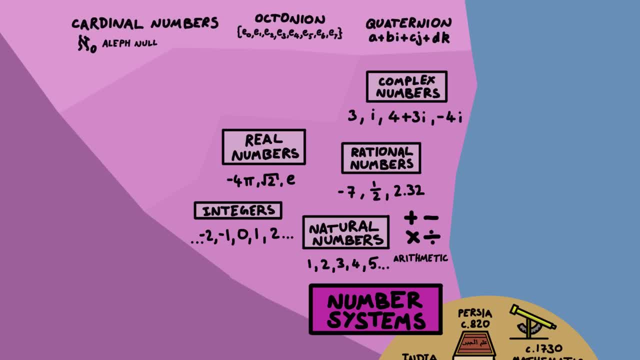 and then complex numbers and a whole bunch of others. Some numbers have interesting properties, like prime numbers or pi or the exponential. There are also properties of these number systems, For example, even though there's an infinite amount of numbers, there are also properties of these numbers systems, For example. 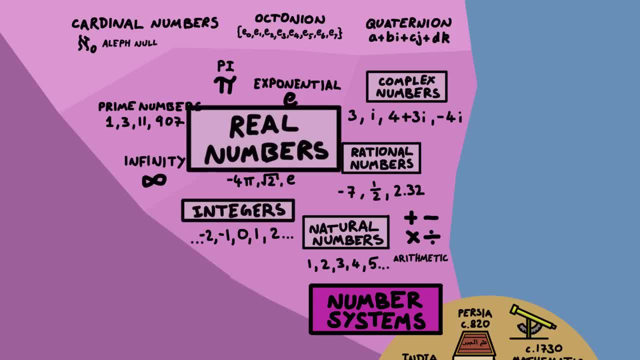 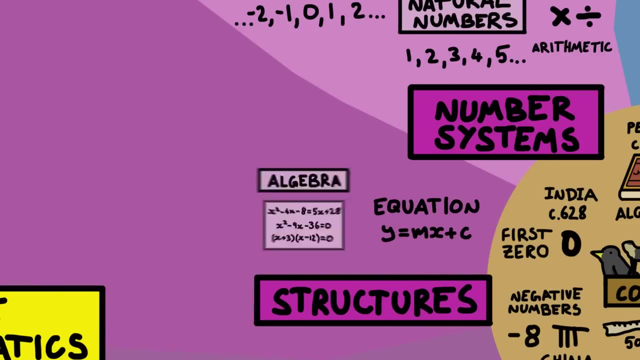 of both integers and real numbers. there are more real numbers than integers, So some infinities are bigger than others. The study of structures is where you start taking numbers and putting them into equations in the form of variables. Algebra contains the rules of how you then manipulate these equations. 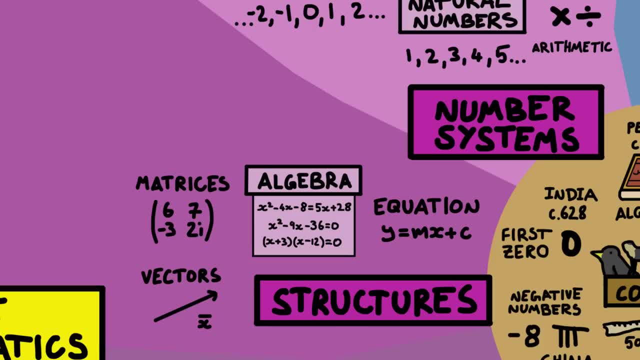 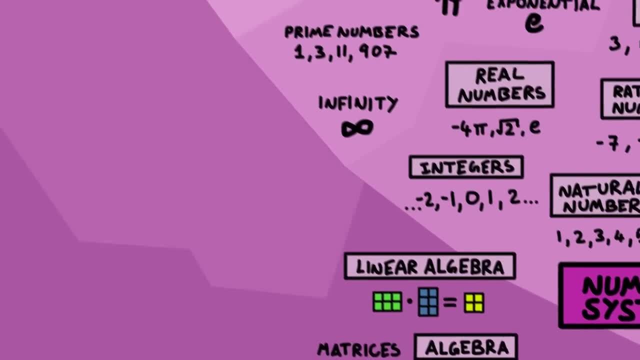 Here you'll also find vectors and matrices, which are multidimensional. numbers and the rules of how they relate to each other are captured in linear algebra. The series of numbers is a large feature in numerical algebra. Number theory studies the features of everything in the last. 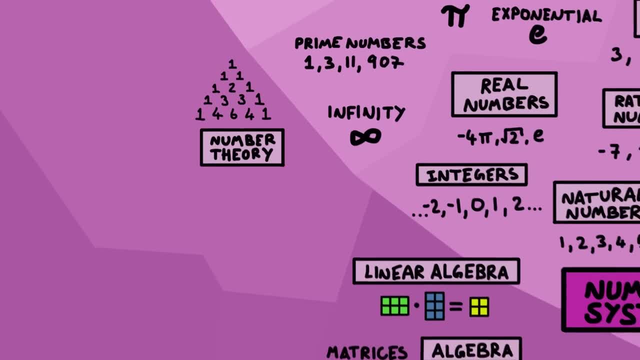 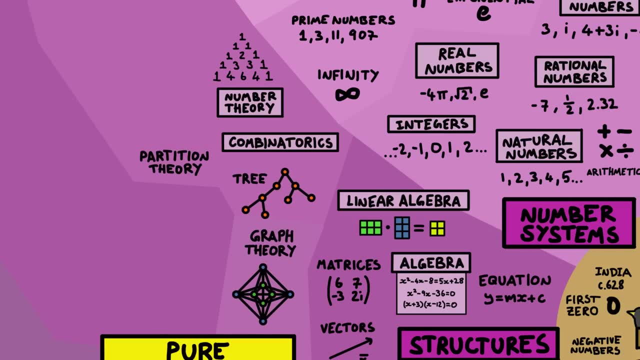 lecture on numbers like the properties of prime numbers. Combinatorics looks at the properties of certain structures like trees, graphs and other things that are made of discrete chunks that you can count. Group theory looks at objects that are related to each other in well groups. 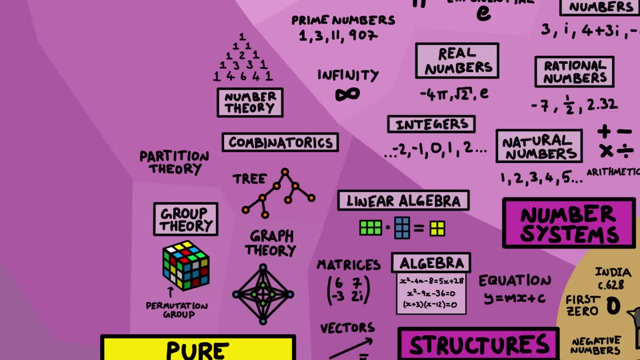 A familiar example is a Rubik's Cube, which is an example of a permutation group, And order theory investigates how to arrange everyone and everything, that means a certain person or property number for the course of the sphere Sheetomenet divided by a number, by a number girdle by a cobra heart compound. 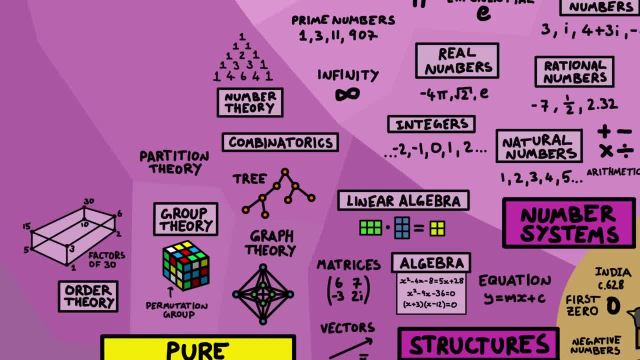 And order theory investigates how to arrange objects by ordination. Sheetomenet alimentos se단 re именно Fantasy, left and right, and señoros ab pedestales y señoros ab~. And order theory investigates how to arrange objects following certain rules. 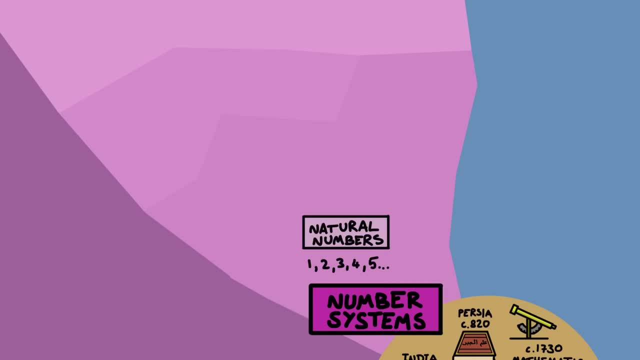 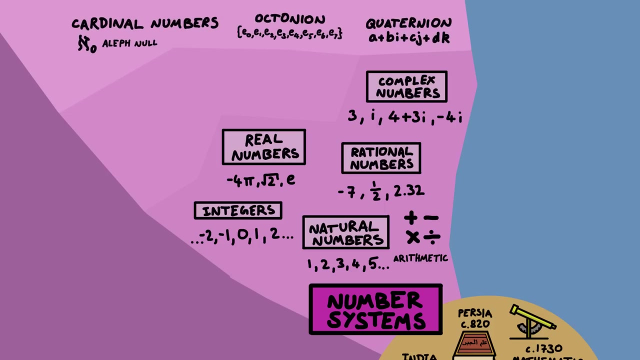 The study of numbers starts with the natural numbers and what you can do with them with arithmetic operations. And then it looks at other kinds of numbers like integers, which contain negative numbers, rational numbers like fractions, real numbers which include numbers like pi, which go off to infinite decimal points, and then complex numbers and a whole bunch of others. Some numbers have interesting properties like prime numbers or pi or the exponential. There are also properties of these number systems. For example, even though there's an infinite amount of numbers in the numbers, there is an infinite amount of numbers in the numbers. So what are the properties of these numbers? Well, there are different properties. 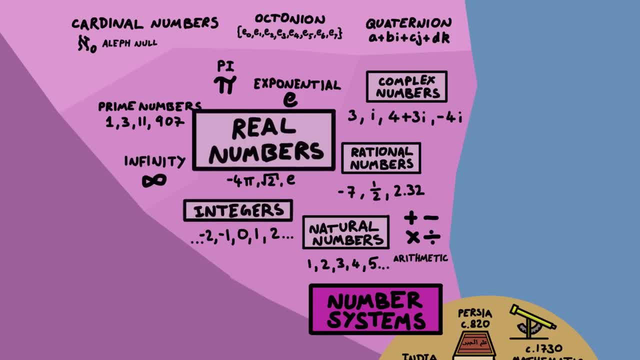 of both integers and real numbers, there are more real numbers than integers, so 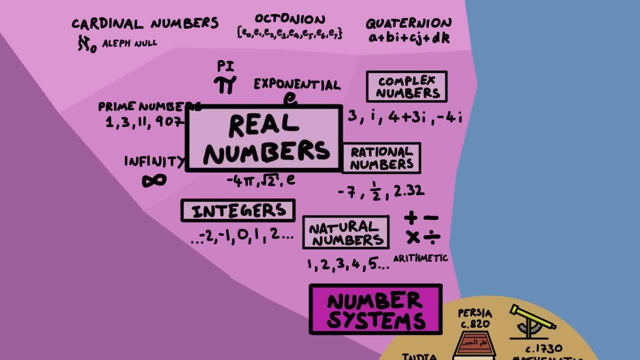 some infinities are bigger than others. 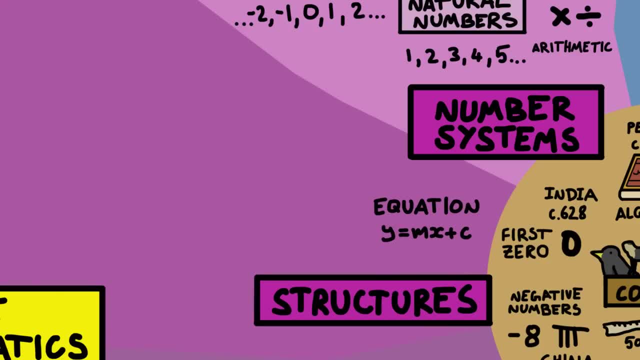 The study of structures is where you start taking numbers and putting them into equations in the form of variables. Algebra contains the rules of how you then manipulate these equations. Here you'll also find vectors and matrices, which are multi-dimensional numbers, and the rules of how they relate to each 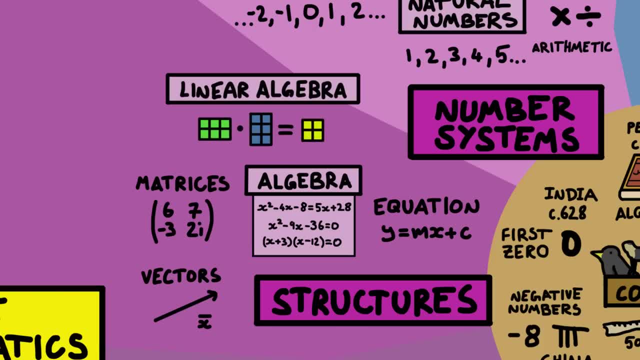 other are captured in linear algebra. 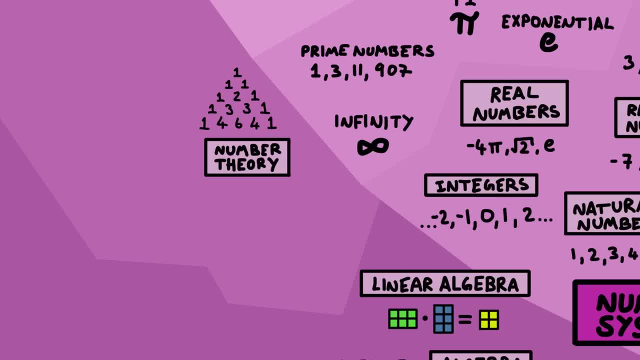 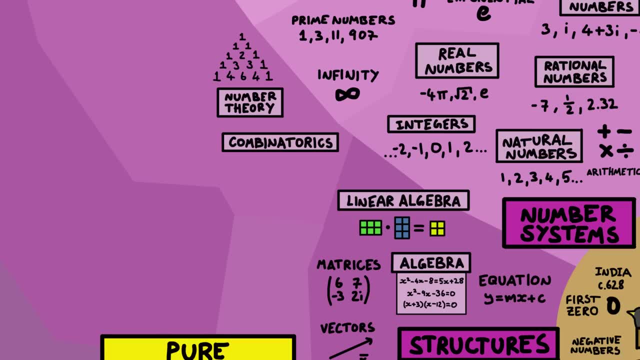 Number theory studies the features of everything in the last section on numbers, like the properties of prime numbers. Combinatorics looks at the properties of certain structures like trees, graphs, and other things that are made of discrete chunks that you can count. Group theory looks at objects that are related to each other in, well, groups. A familiar example is a Rubik's Cube, which is an example of a permutation group. 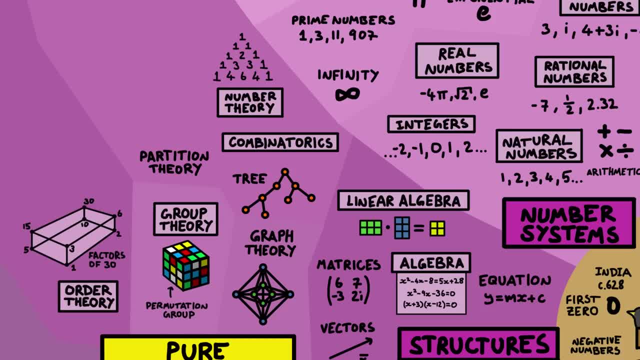 And order theory investigates how to arrange objects following certain rules, like how something is a larger quantity than something else. The natural numbers 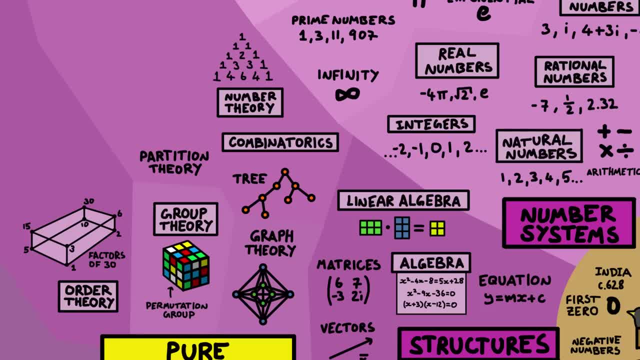 are an example of an ordered set of objects, but anything with any two-way relationship can be ordered. Another part of pure mathematics looks at shapes and 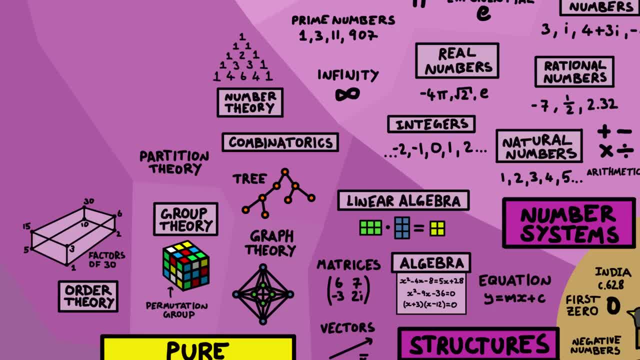 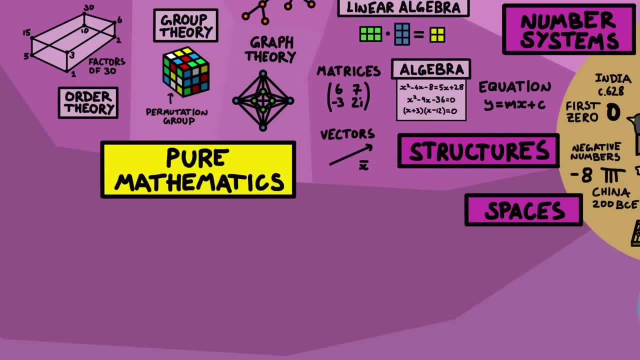 like how something is a larger quantity than something else. The natural numbers are an example of an ordered set of objects, but anything with any two-way relationship can be ordered. Another part of pure mathematics looks at shapes and how they behave in spaces. The origin is in geometry, which includes Pythagoras. 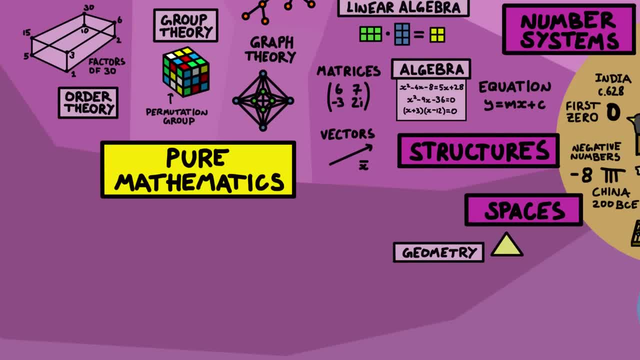 how they behave in spaces. The origin is in geometry, which includes Pythagoras, and is close to trigonometry, which I'm sure we're all familiar with from school. 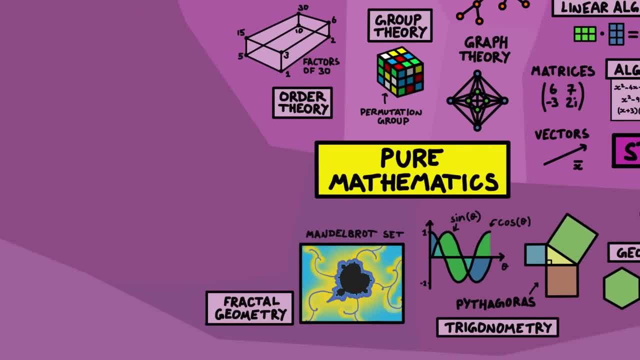 Also, there are fun things like fractal geometry, which are mathematical patterns which are scale-invariant, which means you can zoom into them forever, and they always look kind of the same. Topology looks at different properties of spaces, 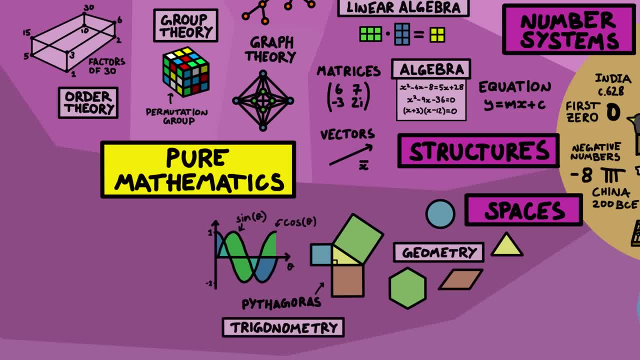 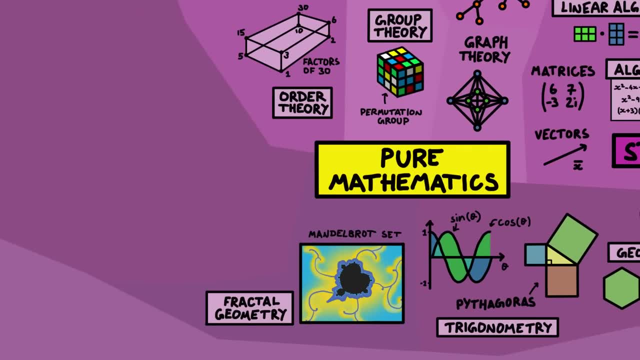 and is close to trigonometry, which I'm sure we're all familiar with from school. Also, there are fun things like fractal geometry, which are mathematical patterns which are scale-invariant, which means you can zoom into them forever and they always look kind of the same. 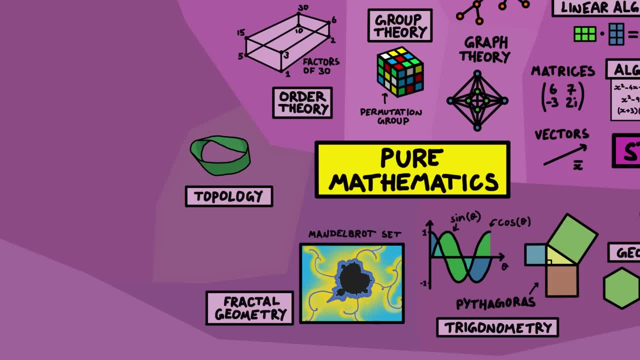 Topology looks at different properties of spaces where you're allowed to continuously deform them, but not tear or glue them. For example, a Mobius strip has only one surface and one edge, whatever you do to it, And coffee cups and donuts are the same thing topologically speaking. 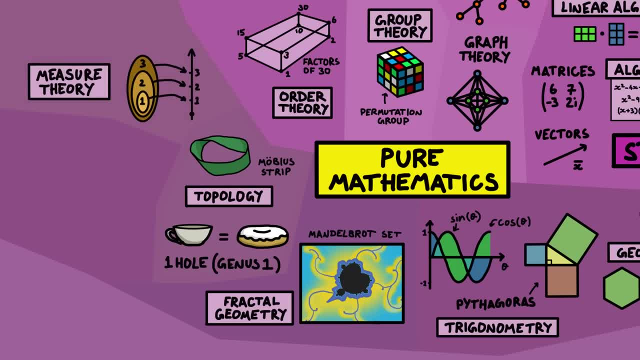 The other part of pure mathematics looks at shapes and how they behave in spaces. Measure theory is a way to assign values to spaces or sets tying together numbers and spaces. And finally, differential geometry looks at the properties of shapes on curved surfaces. 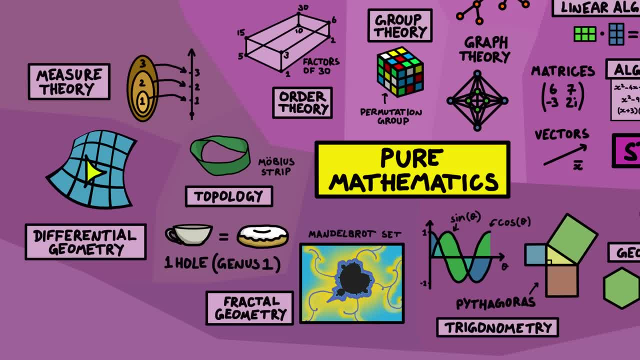 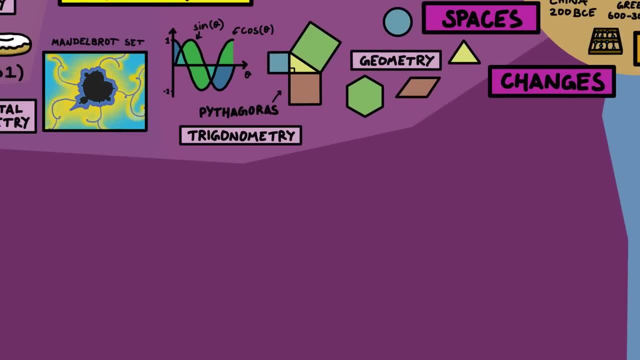 for example, triangles have got different angles on a curved surface. and brings us to the next section, which is changes. The study of changes contains calculus, which involves integrals and differentials, which looks at the area spanned out by functions or the behavior of gradients. 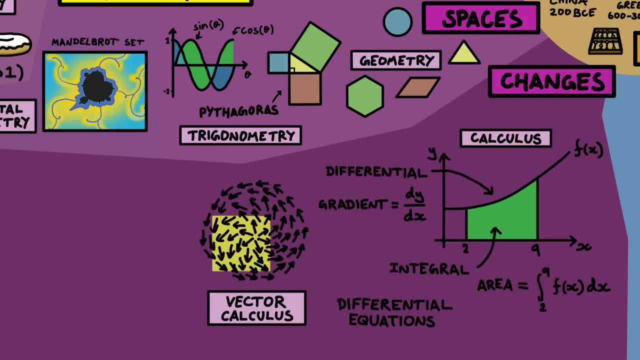 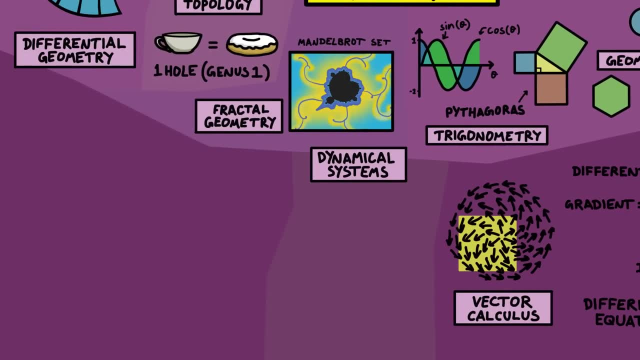 of functions, and vector calculus looks at the same thing, but for vectors. Here we also find a bunch of other areas like dynamical systems, which looks at systems that evolve in time from one state to another, like fluid flows or things with feedback loops. 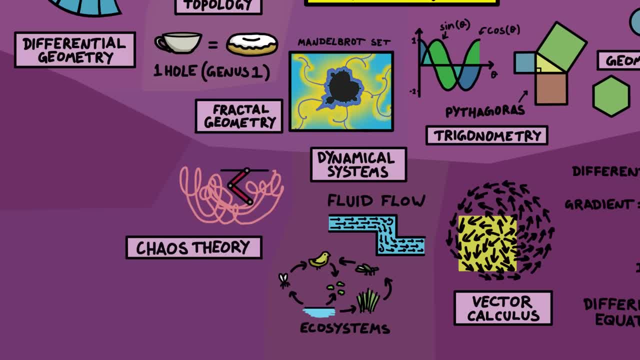 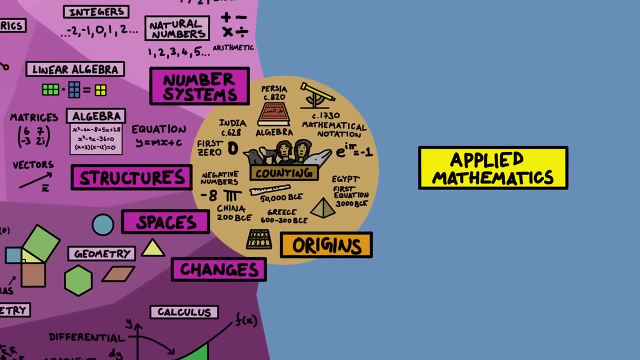 like ecosystems, and chaos theory, which studies dynamical systems that are very sensitive to initial conditions. Finally, complex analysis looks at the properties of functions with complex numbers. This brings us to applied mathematics. At this point, it's probably worth mentioning that everything here is a lot more interrelated than I've 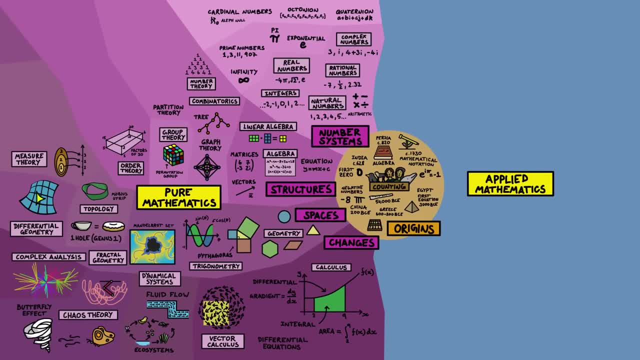 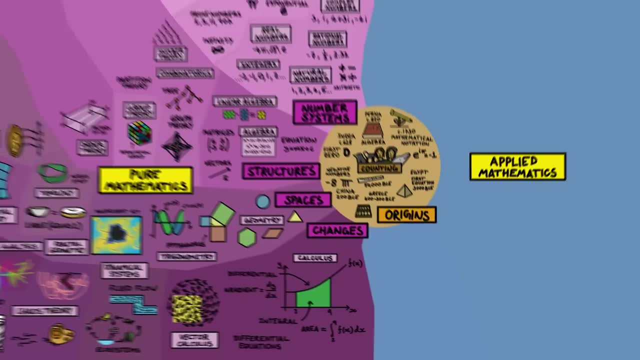 drawn. In reality, this map should look more like a web tying together all the different subjects, but you can only do so much on a two-dimensional plane, so I've laid them out as best I can. Okay, we'll start with physics, which uses just about everything on the left-hand side to some. 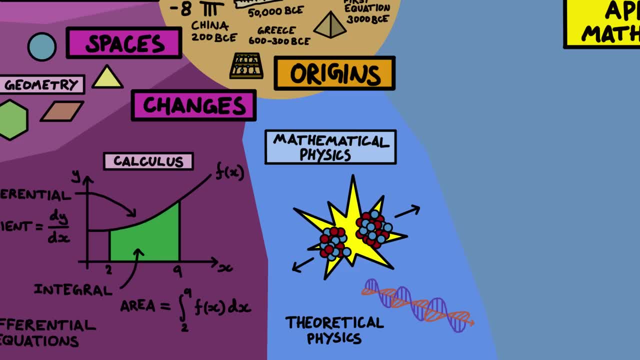 degree. Mathematical and theoretical physics is a very close relationship with pure maths. Mathematics is a very complex and complex field of study, but it's also a very complex field of study, so I'm going to give you a few examples here. Mathematics is also used in the other natural 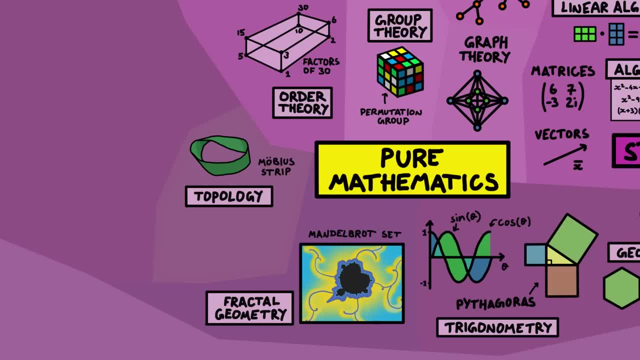 where you're allowed to continuously deform them but not tear or glue them. 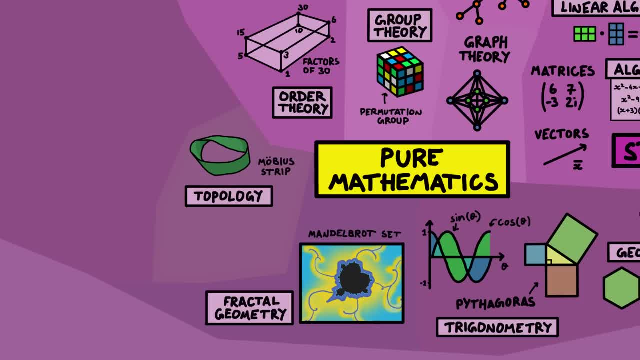 For example, a Mobius strip has only one surface and one edge, whatever you do to 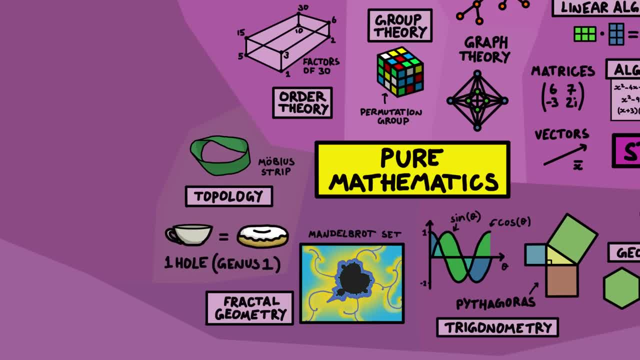 it. And coffee cups and donuts are the same thing, topologically speaking. Measure theory is a way to assign values to spaces or sets, tying together numbers and spaces. 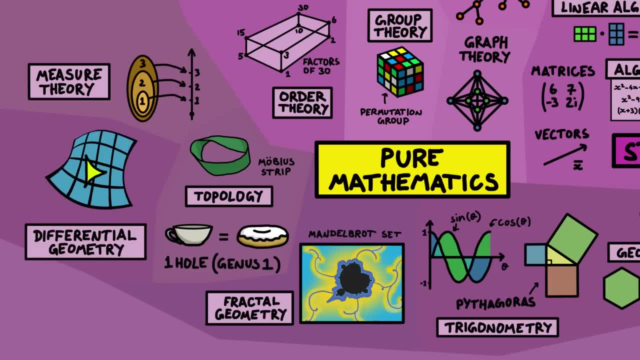 And finally, differential geometry looks at the properties of shapes on curved surfaces, for example triangles have got different angles on a curved surface, and brings us to the next 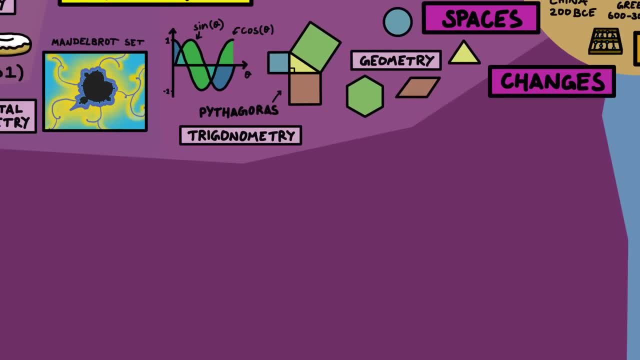 section, which is changes. The study of changes contains calculus, which involves integrals and differentials, which looks at the area spanned out by functions, or the behavior of gradients 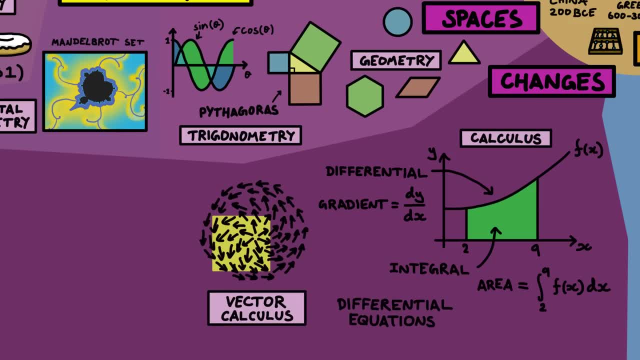 and vectors. And vector calculus looks at the same thing but for vectors. Here we also find a bunch of other areas, like dynamical systems, which looks at systems 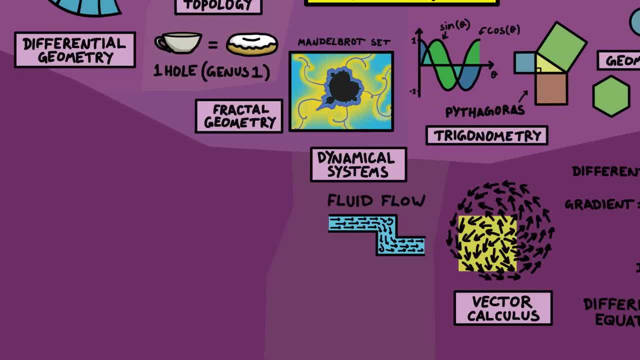 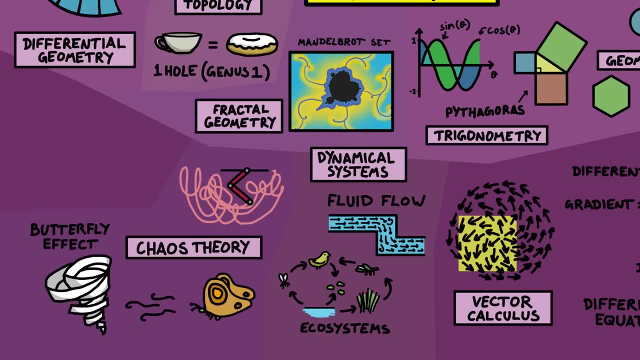 that evolve in time from one state to another, like fluid flows or things with feedback loops like ecosystems. And chaos theory, which studies dynamical systems that are very sensitive 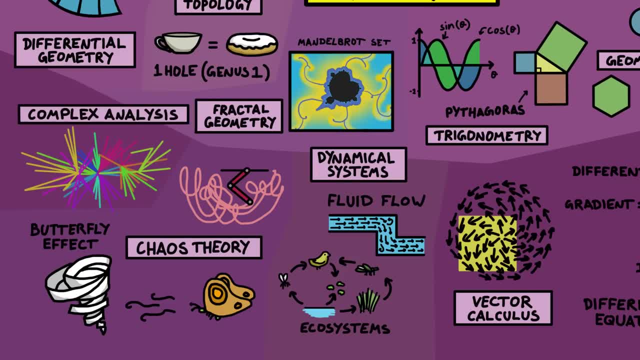 to initial conditions. Finally, complex analysis looks at the properties of functions with complex numbers. 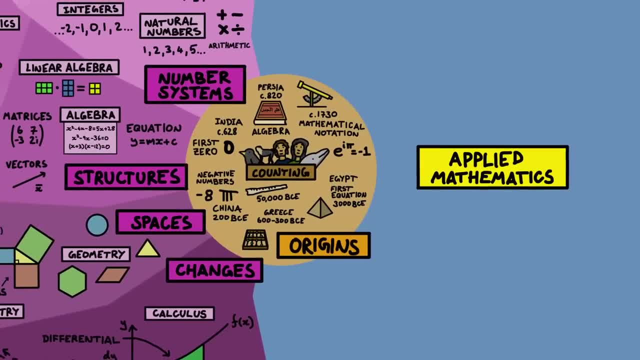 This brings us to applied mathematics. At this point, it's probably worth mentioning that everything here is a lot more interrelated than I've drawn. In reality, this map should 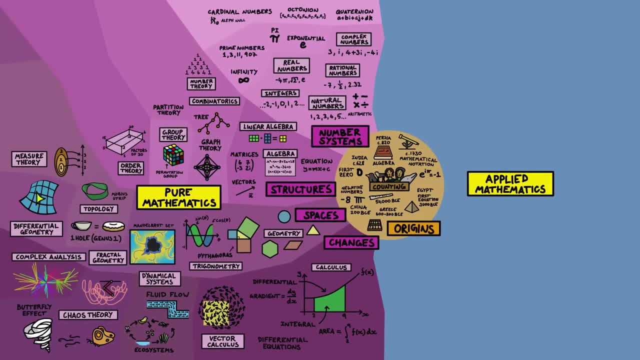 look more like a web tying together all the different subjects, but you can only do so much on a two-dimensional plane, so I've laid them out as best I can. 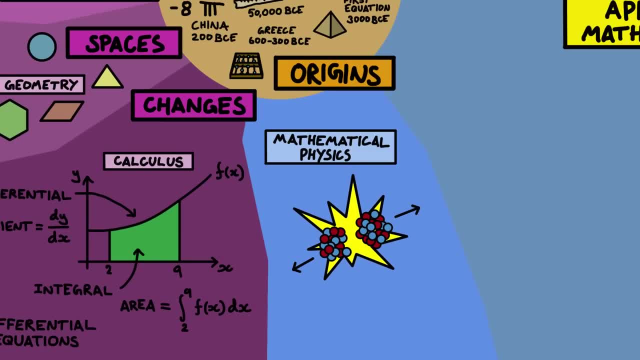 Okay, we'll start with physics, which uses just about everything on the left-hand side to some degree. Mathematical and theoretical physics is a very close relationship with pure maths. Mathematics is also used in the other 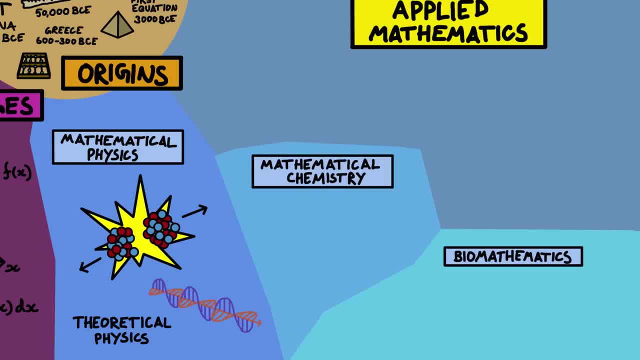 natural sciences, with mathematical chemistry and biomathematics, which look at loads of stuff from modelling molecules to evolutionary biology. Mathematics is also used extensively 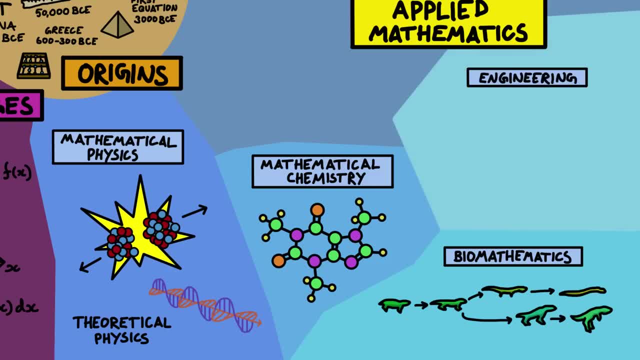 in engineering. Building things has taken a lot of maths since the Egyptians and Babylonian times. Very complex electrical systems, like aeroplanes or the power grid, use methods in dynamical systems, called control theory. 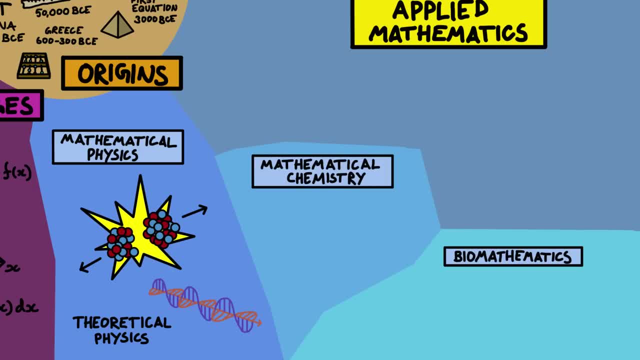 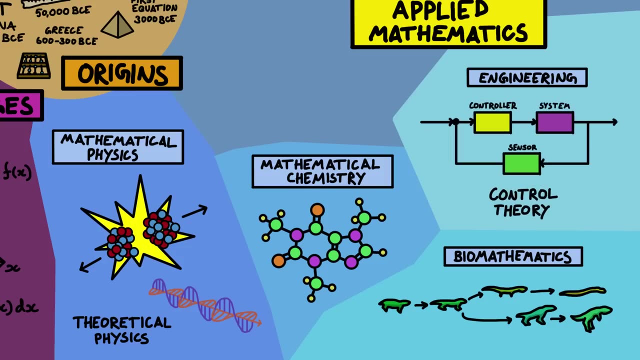 sciences, with mathematical chemistry and biomathematics, which look at loads of stuff from modelling molecules to evolutionary biology. Mathematics is also used extensively in engineering: Building- things has taken a lot of maths since the Egyptians and Babylonian times- Very complex electrical systems like aeroplanes or the power grid. 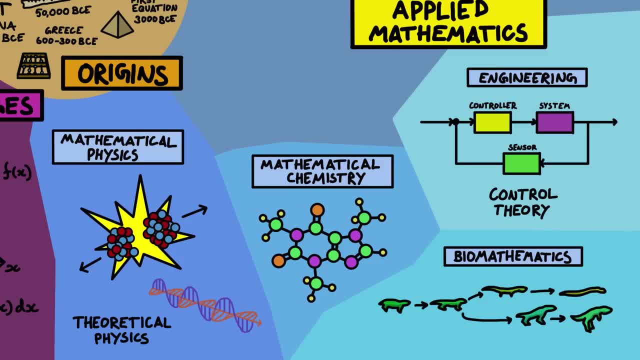 use methods in dynamical systems called control theory. Numerical analysis is a maths theory that has been used extensively in engineering building things and very complex electrical systems like aeroplanes or the power grid. use methods in dynamical systems called control theory. 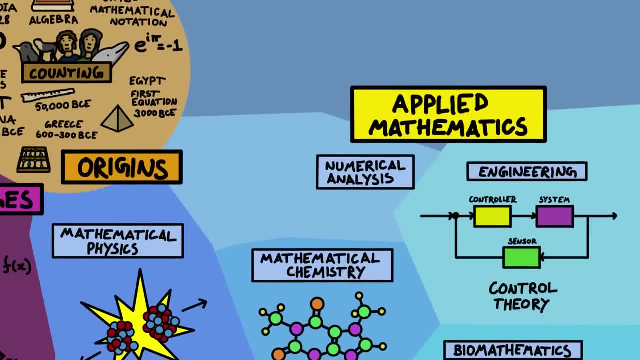 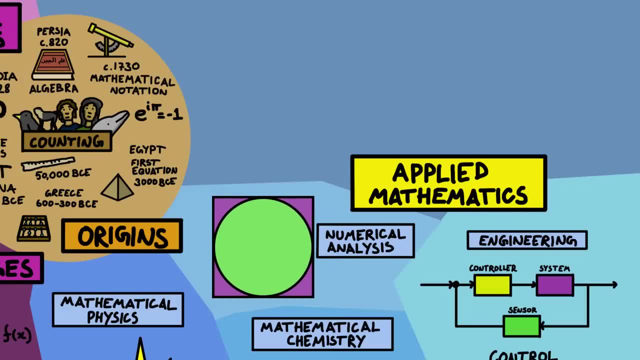 Numerical analysis is a mathematical tool commonly used in places where mathematics becomes too complex to solve completely. So instead you use lots of simple approximations and combine them all together to get good, approximate answers. For example, if you put a circle inside a square, throw darts at it. 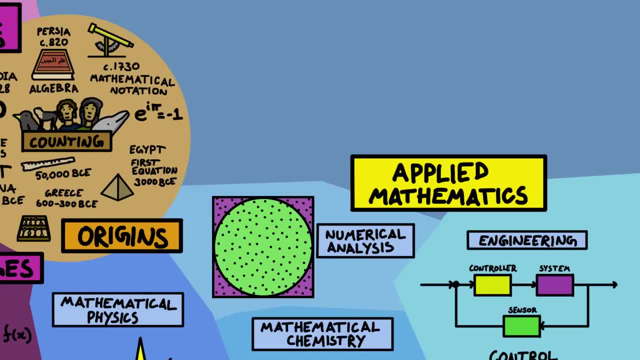 and then compare the number of darts in the circle and the square portion, you can approximate the value of pi. But in the real world numerical analysis is done on huge computers. Game theory looks at what the best choices are, given a set of rules and rational players. 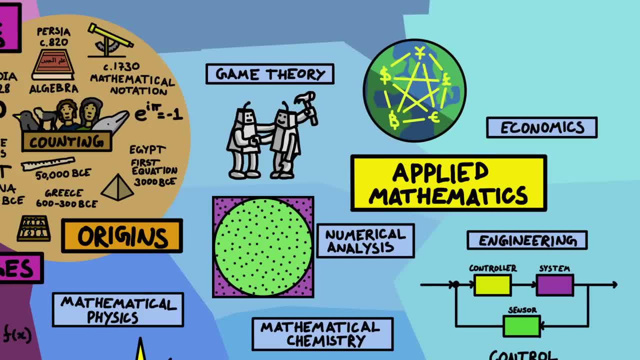 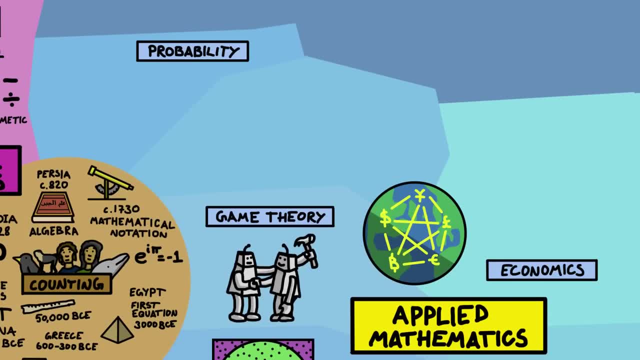 and it's used in economics, when the players can be intelligent but not always, and other areas like psychology and biology. Probability is the study of random events like coin tosses or dice or humans, and statistics is the study of large collections of random processes or the organization. 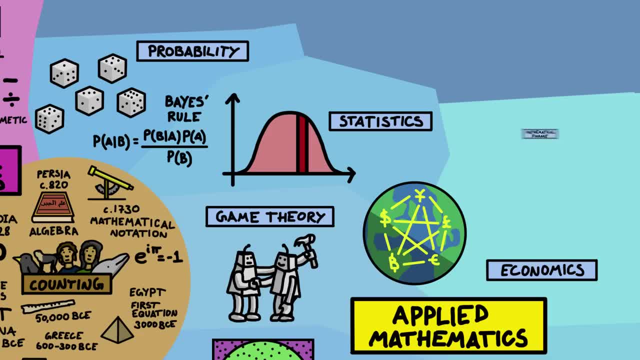 and analysis of data. This is obviously related to mathematical finance, where you want to model financial systems in the mathematical field And what you're looking for is more of a mathematical systems can get an edge to win all those fat stacks. Related to this is optimization, where 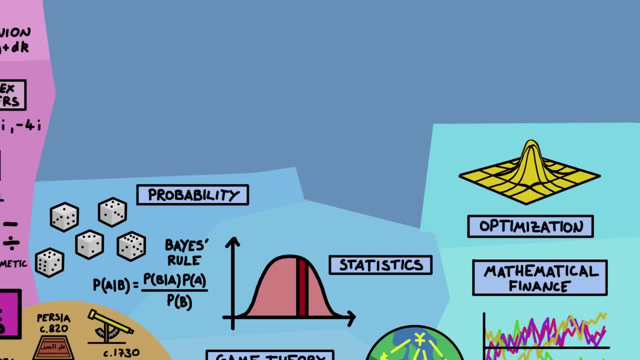 you're trying to calculate the best choice amongst a set of many different options or constraints, which you normally visualize as trying to find the highest or lowest point of a function. Optimization problems are second nature to us humans and we do them all the time, trying to get the best value for money or trying to maximize our happiness in some way. 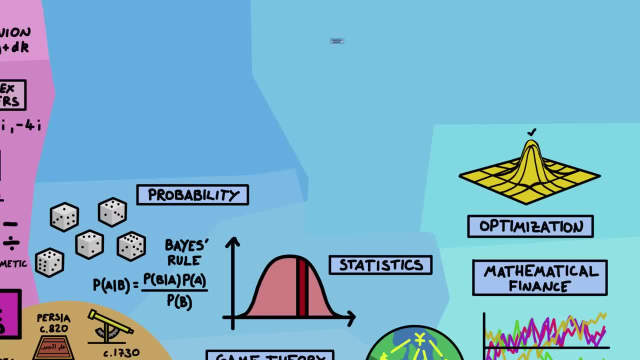 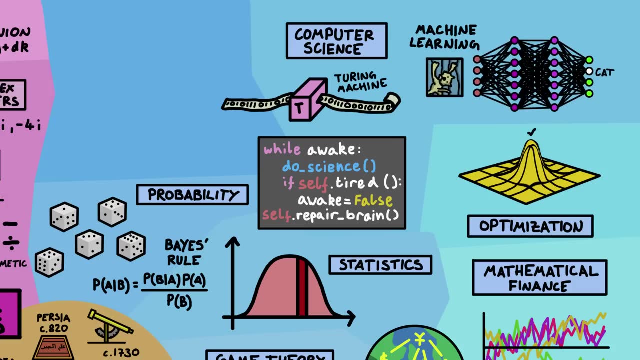 Another area that's very deeply related to pure mathematics is computer science, and the rules of computer science were actually derived in pure maths and is another example of something that was worked out way before programmable computers were built: Machine learning- the creation of intelligent computer systems, uses many areas in mathematics, like linear algebra optimization. 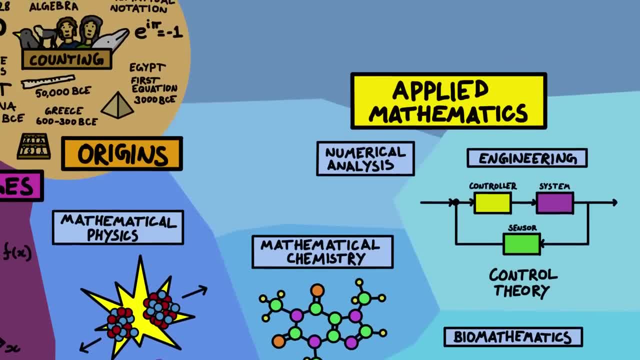 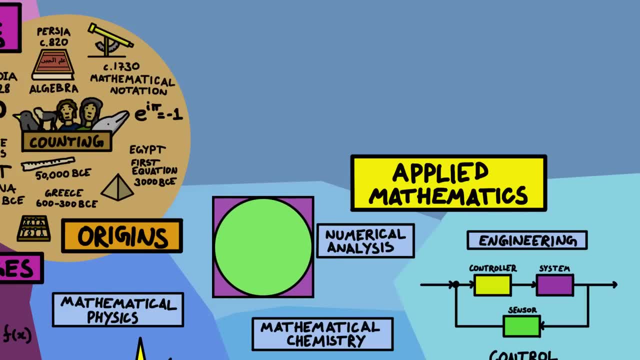 Numerical analysis is a mathematical tool commonly used in places where mathematics becomes too complex to solve completely. So instead you use lots of simple approximations and combine them all together to get good approximate answers. For example, if you put a circle inside a square, throw darts 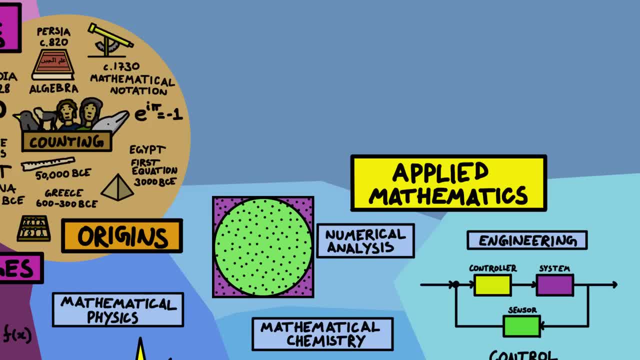 at it, and then compare the number of darts in the circle and the square portion, you can approximate the value of pi. But in the real world, numerical analysis is done on 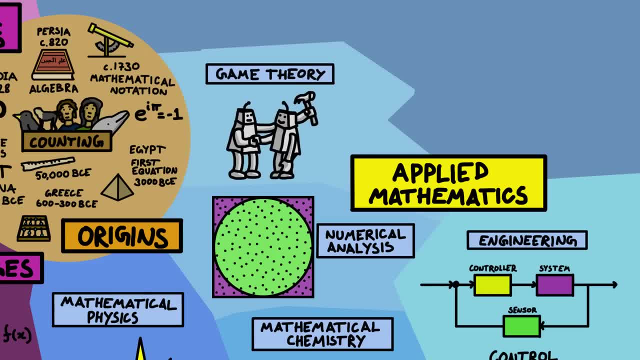 huge computers. Game theory looks at what the best choices are, given the number of darts in the circle, and the number of darts in the circle, and the number of darts in the circle. 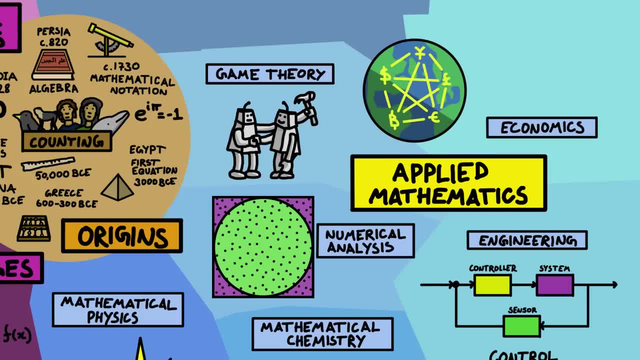 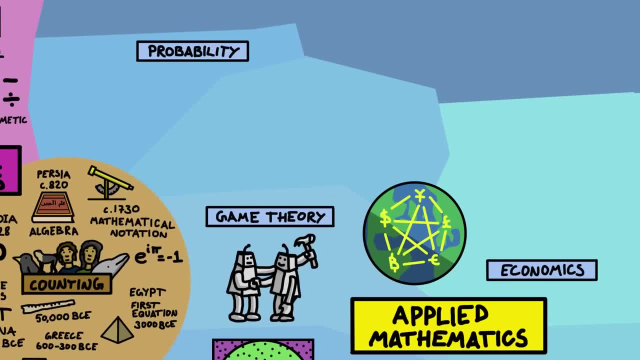 Mathematics is also used in economics, where the players can be intelligent, but not always, and other areas like psychology and biology. Probability is the study of random events 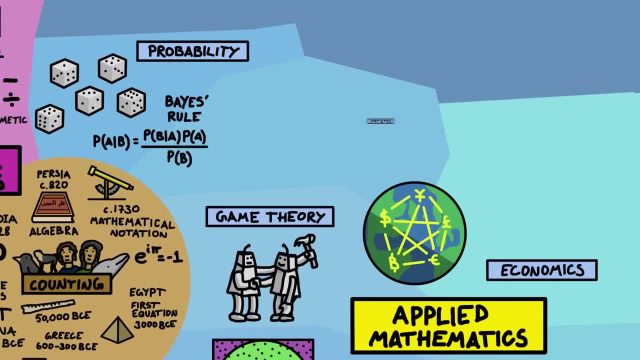 like coin tosses, or dice, or humans. And statistics is the study of large collections of random processes, or the organisation and analysis of data. This is obviously related 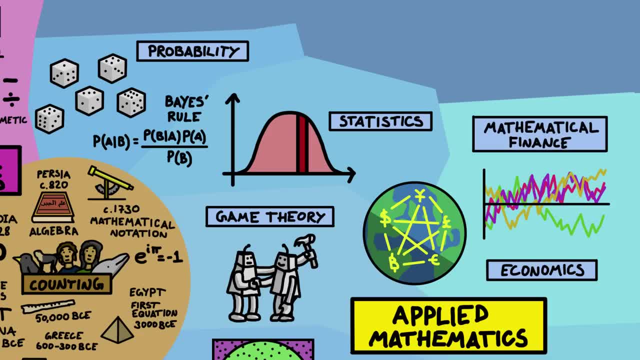 to mathematical finance, where you want to model financial systems and get an edge to win all those fat stacks. 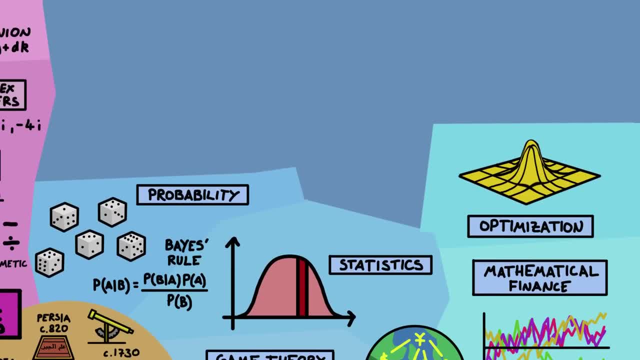 Related to this is optimisation, where you're trying to calculate the best choice amongst a set of many different options or constraints, which you can normally visualise as trying to find the highest or lowest point of a function. Optimisation problems are second nature to 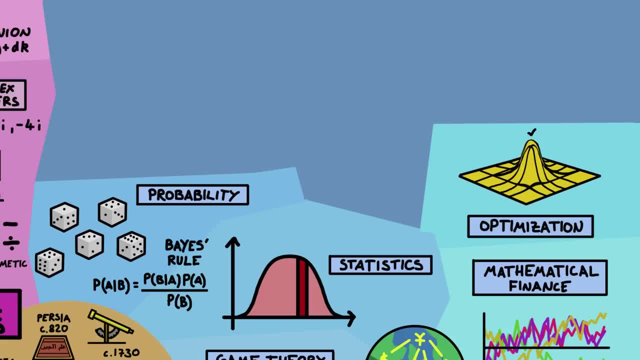 us humans, and we do them all the time, trying to get the best value for money, or trying to maximise our happiness in some way. 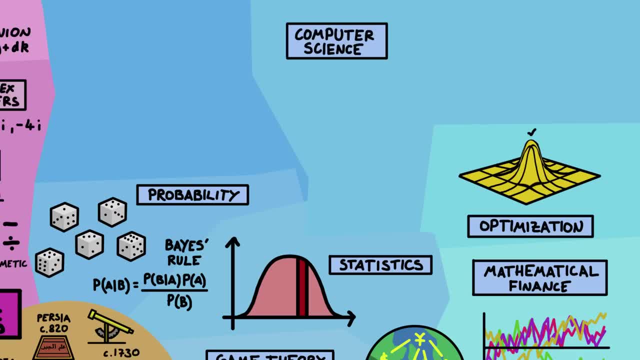 Another area that's very deeply related to pure mathematics is computer science, and the 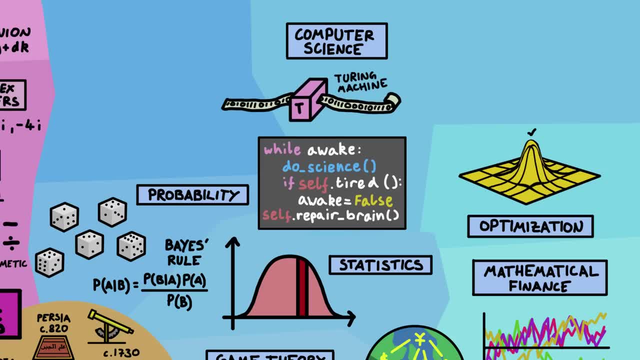 rules of computer science were actually derived in pure maths, and is another example of something that was worked out way before programmable computers were built. Machine learning, the 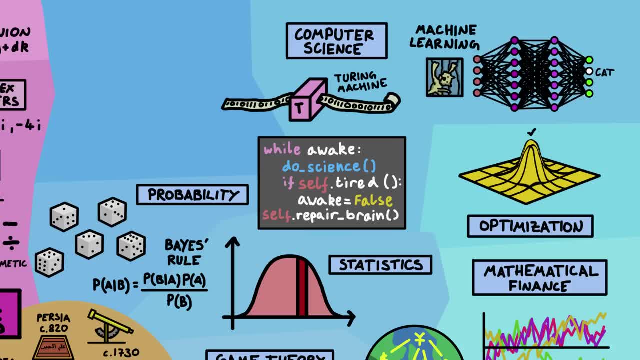 creation of intelligent computer systems, uses many areas in mathematics, like linear algebra, optimisation, dynamical systems, and probability. 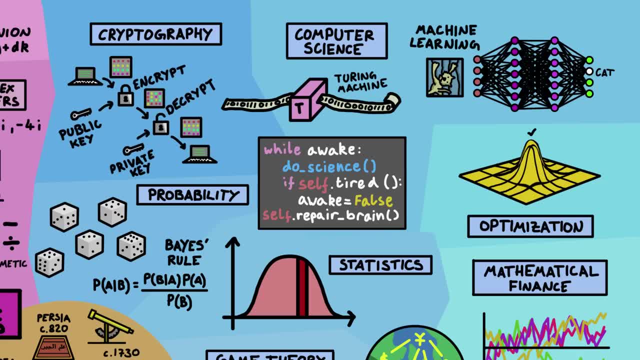 And finally, the theory of cryptography is very important to computation, and uses a lot of pure maths, like combinatorics and number theory. So that covers the main sections of pure and applied mathematics. 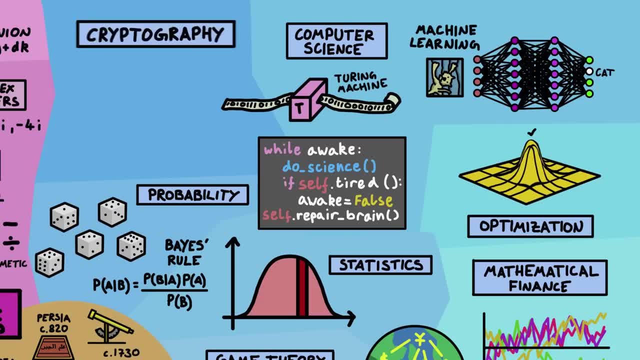 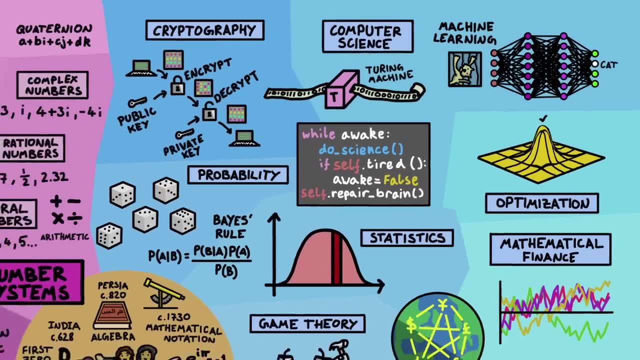 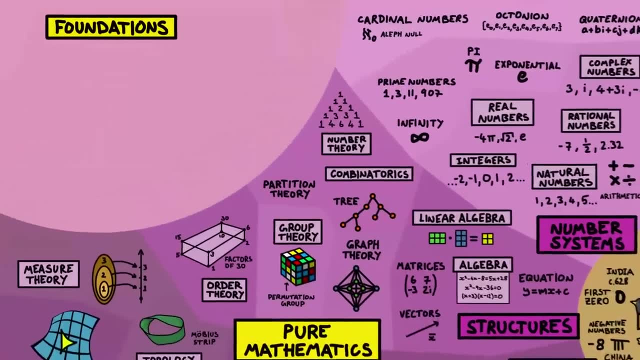 dynamical systems and probability. And finally, the theory of cryptography is very important to computation and uses a lot of pure maths like computation and computation, combinatorics and number theory. So that covers the main sections of pure and applied mathematics, but I can't end without looking at the foundations of mathematics. This area tries to work out the 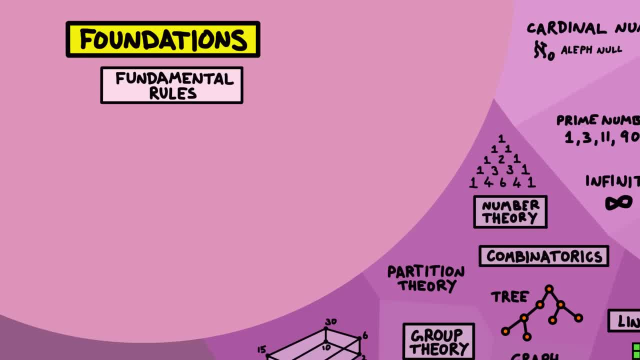 properties of mathematics itself and asks what the basis of all the rules of mathematics is. Is there a complete set of fundamental rules, called axioms, which all of mathematics comes from, and can we prove that it's all consistent with itself? Mathematical logic set theory. 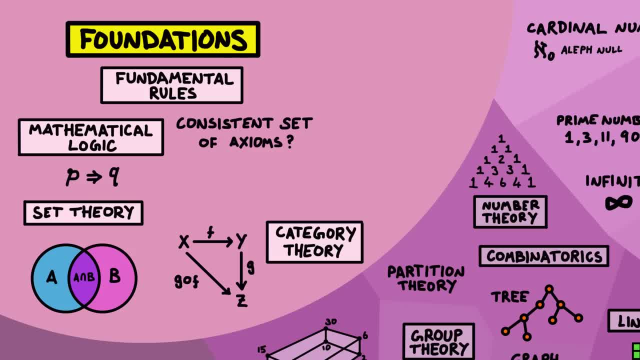 and category theory try to answer this, and a famous result in mathematical logic are Gödel's incompleteness theorems, which for most people means that mathematics does not have a complete and consistent set of axioms, which means that it's all kind of made up by us humans, Which is weird. 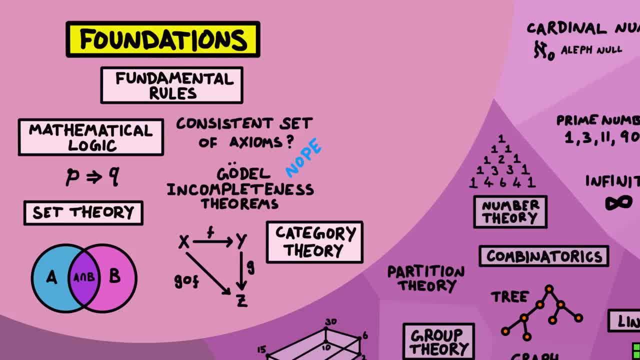 seeing as mathematics explains so much stuff in the universe so well, why would a thing made up by humans be able to do that? That is a deep mystery. right there We also have the theory of computation, which looks at different models of computing and how efficiently. 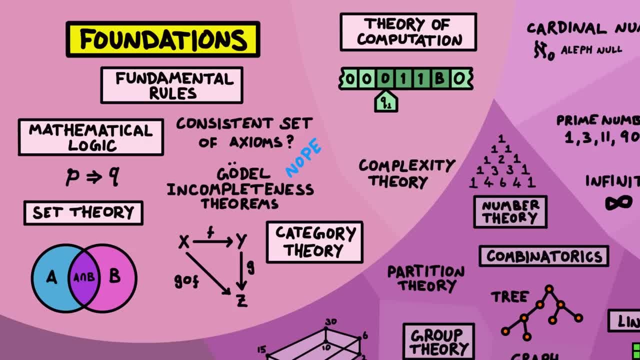 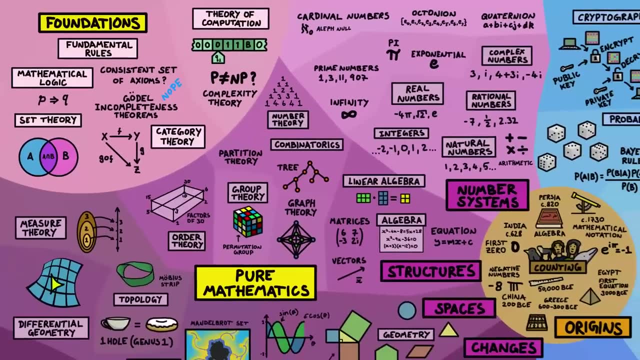 they can solve problems, and contains complexity theory, which looks at what is and isn't computable and how much memory and time you would need, which, for most interesting problems, is an insane amount. So that is the map of mathematics. Now, the thing I've loved most about learning maths is that 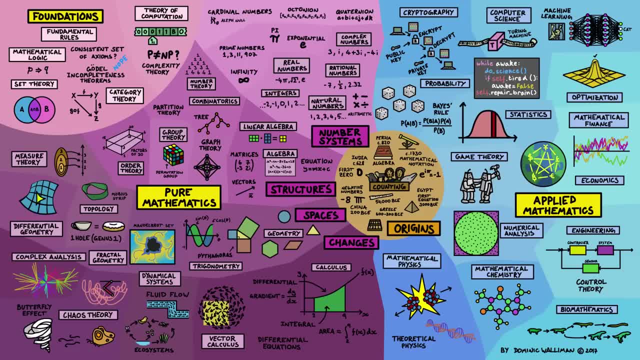 feeling you get where something that seemed so confusing finally clicks in your brain and everything makes sense, Like an epiphany moment, kind of like seeing through the matrix. In fact, some of my most satisfying intellectual moments have been understanding some part of mathematics and then feeling like I had a 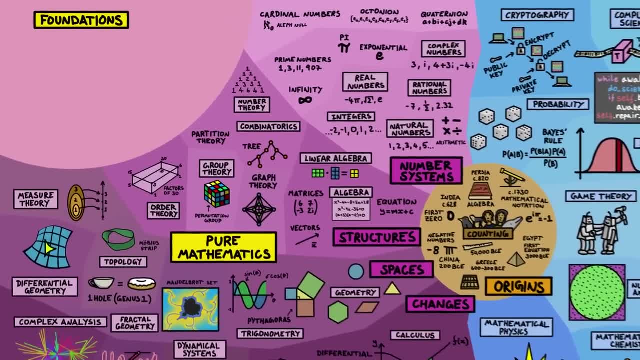 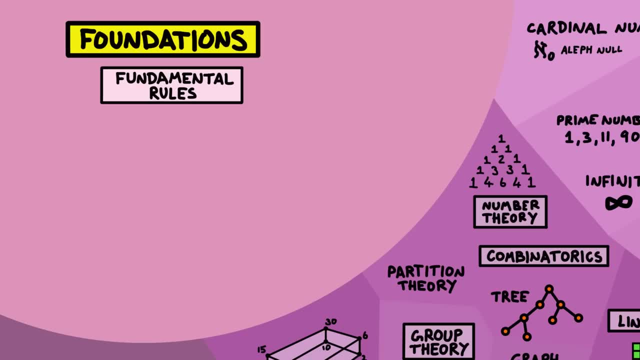 But I can't end without looking at the foundations of mathematics. This area tries to work out the properties of mathematics itself, and asks what the basis of all the rules of mathematics is. Is there a complete set of fundamental rules, called axioms, which all of mathematics comes from? And can we prove that it's all consistent with itself? 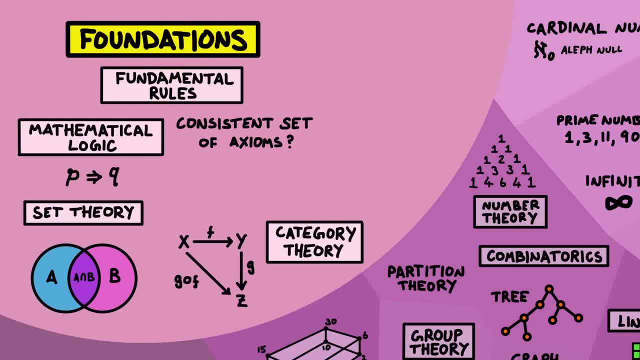 Mathematical logic, set theory, and category theory try to answer this, and a famous result in mathematical logic are GERDs. Mathematical logic, set theory, and category theory try to answer this, and a famous result in mathematical logic are GERDs. Mathematical logic, set theory, and category theory try to answer this, and a famous result in mathematical logic are GERDs. 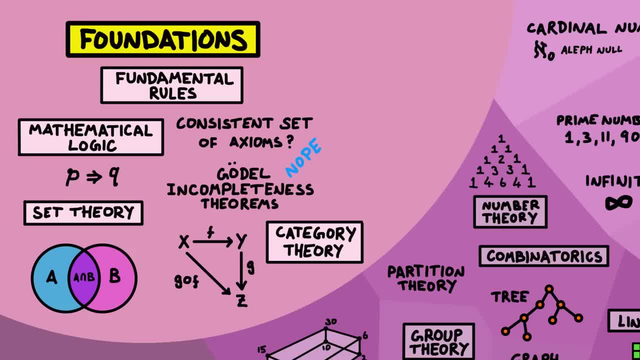 For most people, the biggest part is that mathematics does not have a complete and consistent set of axioms, and that means it's all kind of made up by the humans. 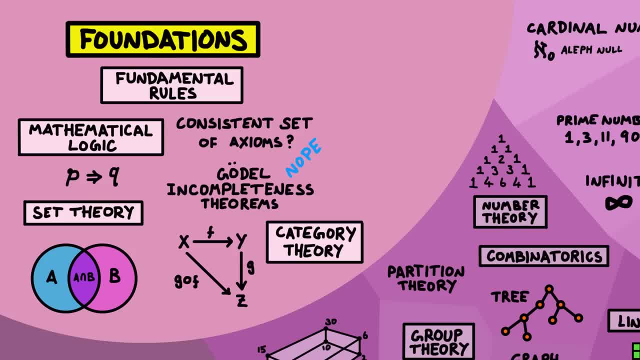 Which is weird, because math quality is bit odd, and can explain so much stuff in the universe so well… Why would a thing made up by humans be able to do that? 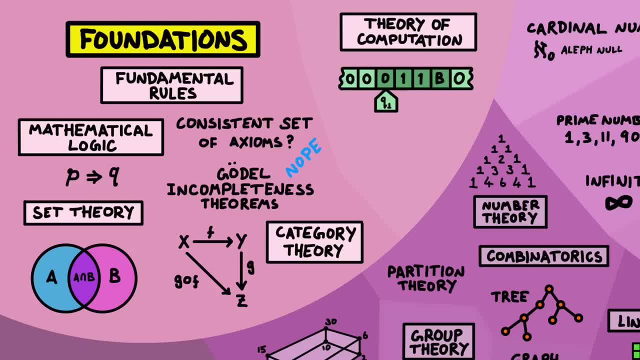 We also have the theory of computation, which looks at different models of computing, and how efficiently a machine is coupled together to factor in the, overall formula and the value of computational statement. 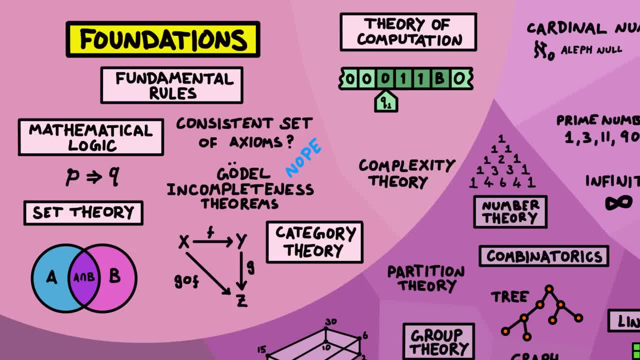 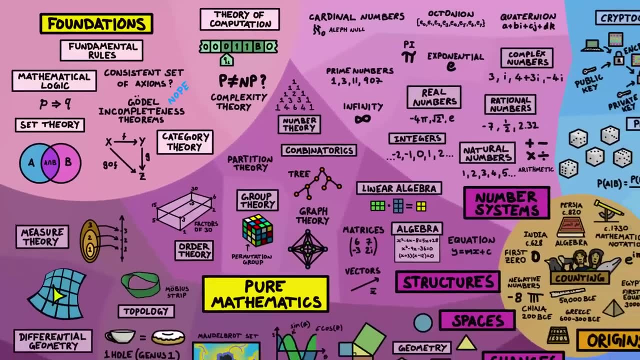 they can solve problems and contains complexity theory, which looks at what is and isn't computable and how much memory and time you would need, which for most interesting problems is an insane amount. So that is the map of mathematics. Now the thing I've loved most about learning 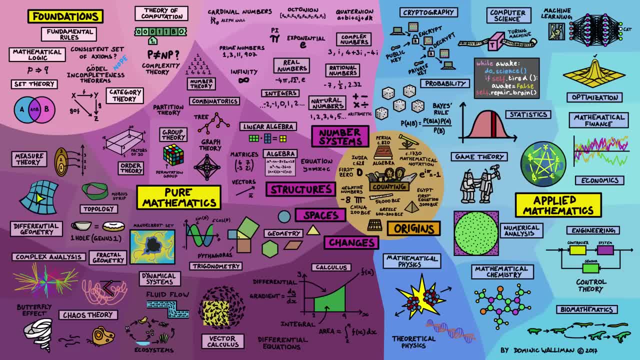 maths is that feeling you get where something that seemed so confusing finally clicks in your brain and everything makes sense, like an epiphany moment, kind of like seeing through the matrix. 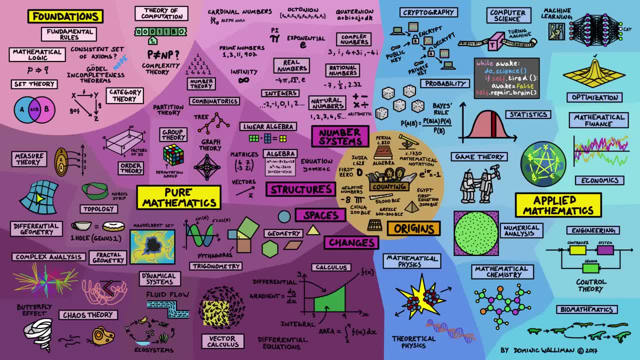 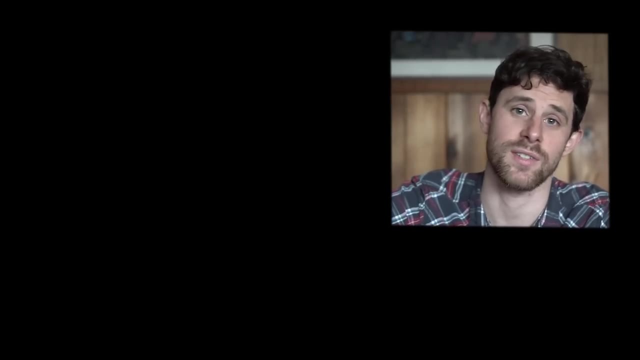 In fact, some of my most satisfying intellectual moments have been understanding some part of mathematics and then feeling like I had a glimpse at the fundamental nature of the universe in all of its symmetrical wonder. It's great. I love it. Making a map of mathematics was the most popular request I got, which I was really happy about because I love maths and it was great to see so much interest in it. So I hope you enjoyed it. Obviously, there's only so much I can say about it, but I hope you enjoyed it. And if you enjoyed it, please do give it a thumbs up. And I'll see you in the next video. Bye. 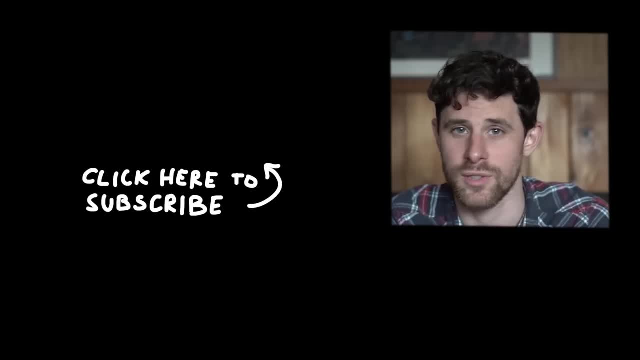 I don't know if I can get into this time frame, but hopefully I've done the subject justice and you found it useful. So there'll be more videos coming from me soon. Here's all the regular things 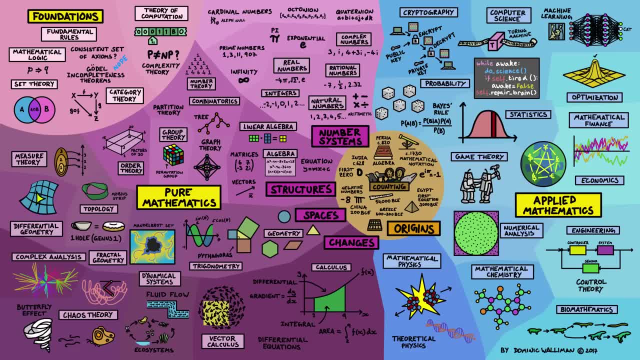 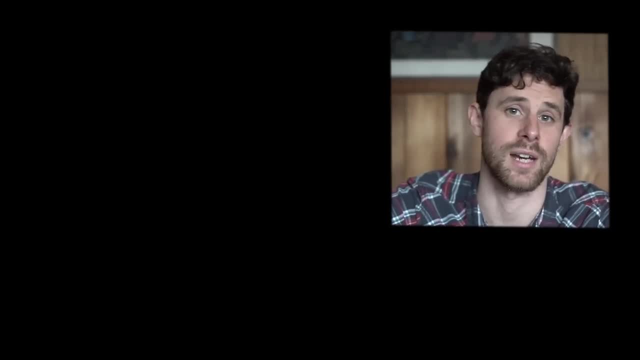 glimpse at the fundamental nature of the universe in all of its symmetrical wonder. It's great, I love it. Making a map of mathematics was the most popular request I got, which I was really happy about because I love maths and it was great to see so much interest in it. 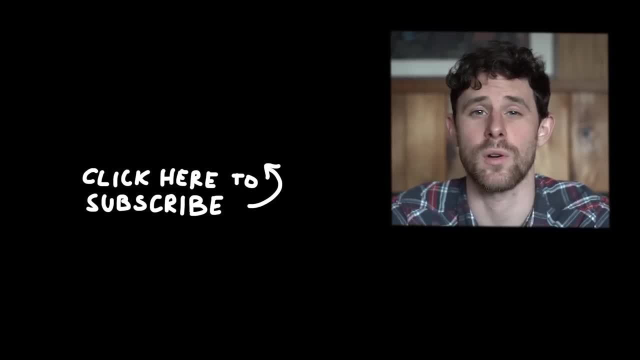 So I hope you enjoyed it. Obviously, there's only so much I can get into this time frame, but hopefully I've done the subject justice and you found it useful, So there'll be more videos coming from me soon. Here's all the regular things, and it was my pleasure See you next time.